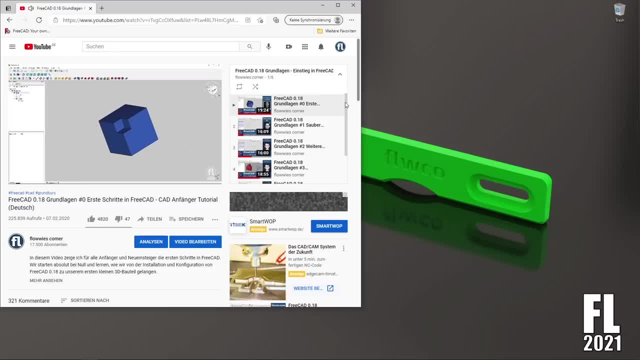 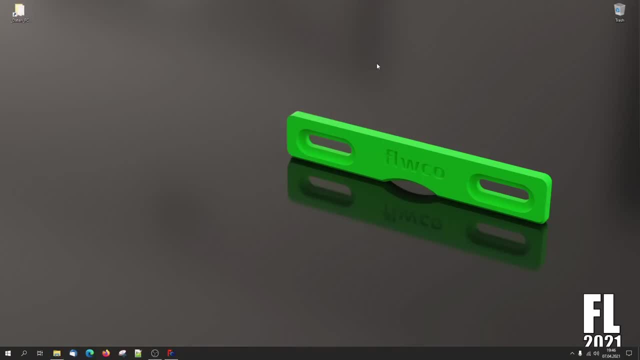 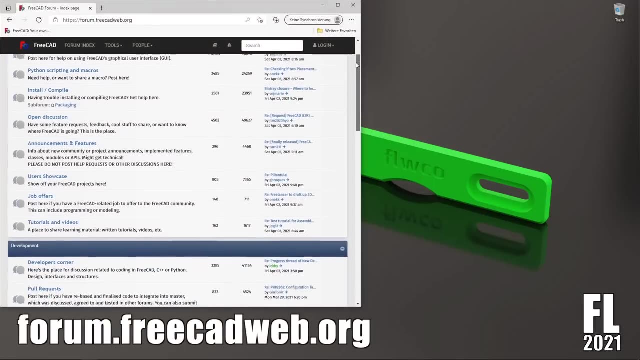 this course available for my international audience here in the FreeCAD Academy. FreeCAD itself is an open source community, so the community is very important for FreeCAD. You can participate in the community by using the forum, where you can ask for help or show your own personal FreeCAD project If you want to participate more in the 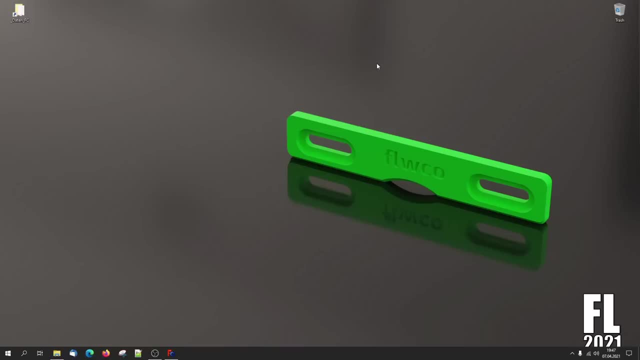 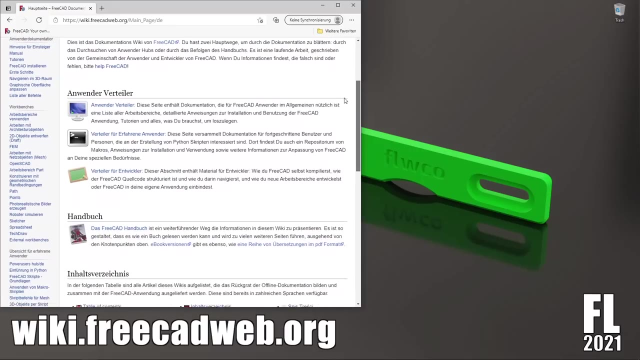 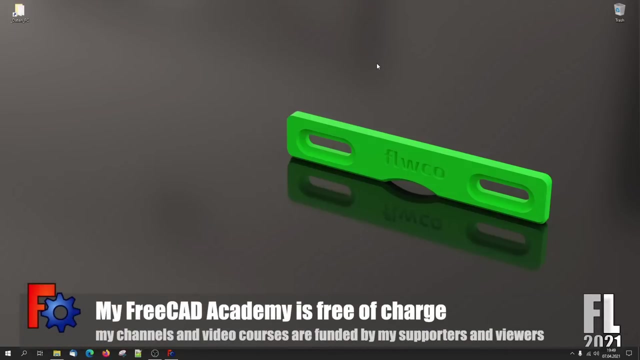 FreeCAD community. you could probably help translating or upgrading the documentation, the so-called FreeCAD Wiki, and there are several other ways to help improving and contributing to FreeCAD. This course is funded by generous donations from my FreeCAD community, so I get paid by the viewers, so I don't have to make deals with companies or advertisements here. 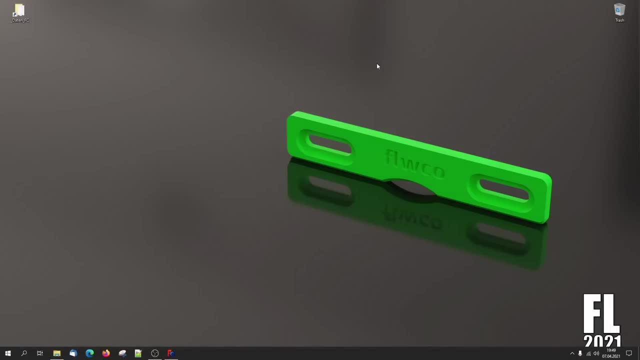 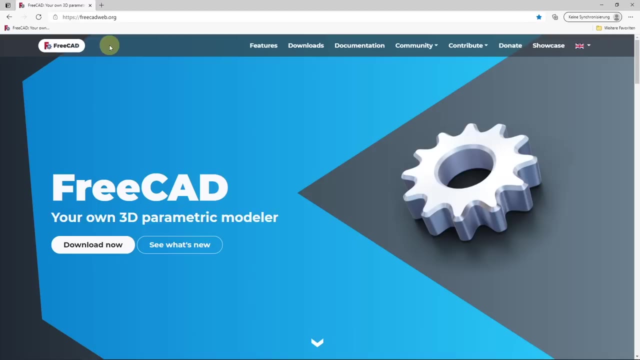 For products or affiliate links and other stuff. So it's completely free and funded by the viewers. And now let's start this video course. The first thing you should do in order to start with FreeCAD is to go to the website freecadweborg. This is FreeCAD's official website and the starting point. 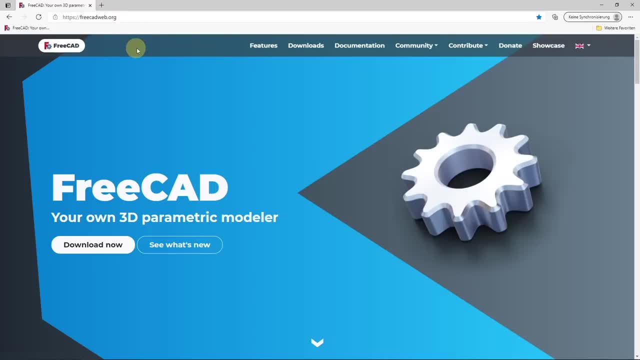 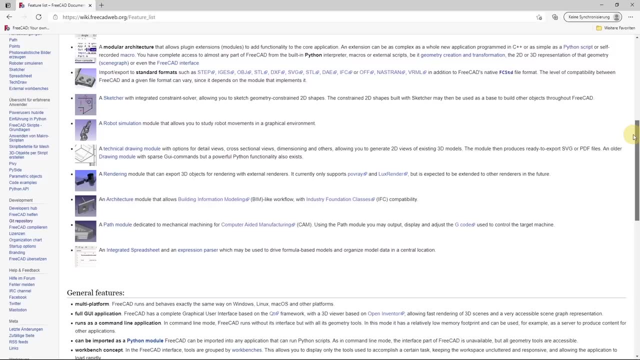 for you in your journey with FreeCAD. What do we have on the website? We have a features list. you can click on this and see all the wonderful features that are currently in FreeCAD and that are currently under development. We have the downloads. I will talk about this later. 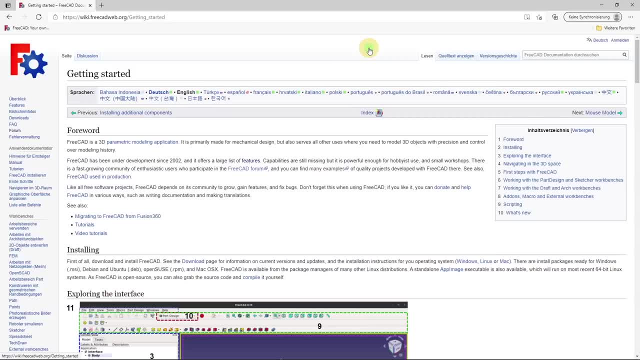 This is one of the most important tabs overall: the documentation, or the so-called Wiki, where you find all the information how FreeCAD works, tutorials. It's a great manual on all the specific tools within FreeCAD, about the specific workbenches, and there is so much information. 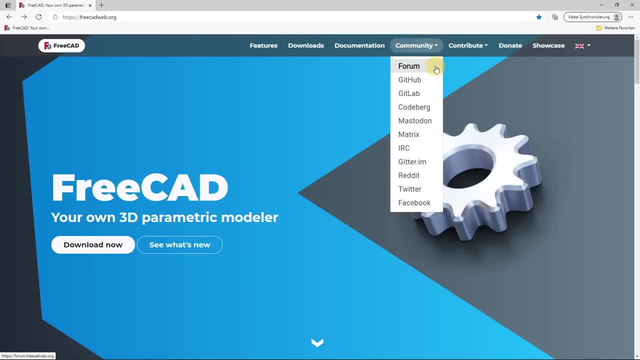 in here. Next thing is the community. Most important in the community is the forums, but there are a lot of other ways to interact with other FreeCAD users. You will learn how to contribute to FreeCAD, how you can help, how you can. 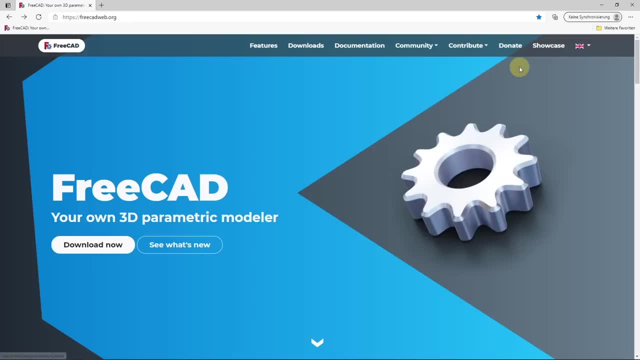 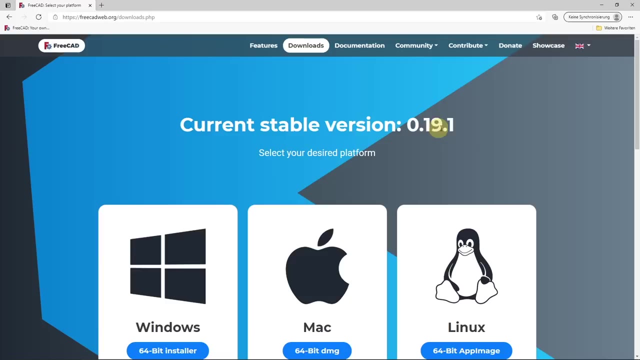 track bugs, how you can contribute to the Wiki, you can donate to the FreeCAD organization and you will have a showcase on some nice models that have been built within FreeCAD. So we switch to downloads, and under downloads we will find the current stable version is the 19.1 and we have 3.1. 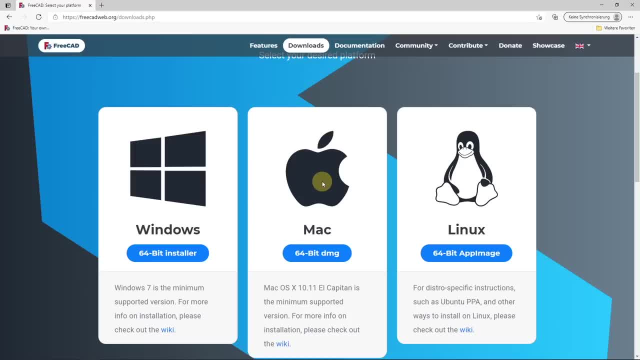 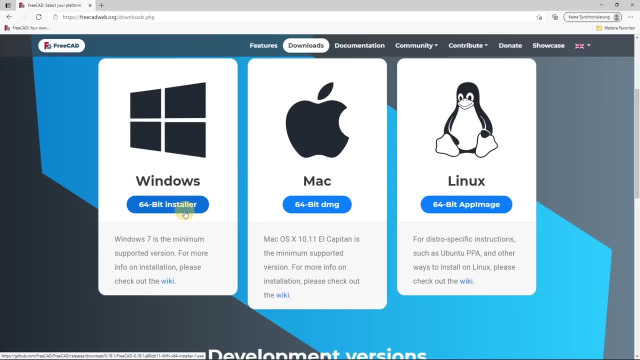 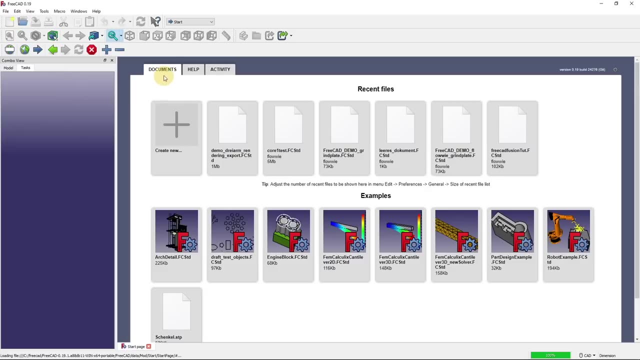 This is where we can start the installation of FreeCAD, and that's Windows, MacOS and Linux. I will continue with this video after the installation in Windows 10.. See you there. Here we are in the fresh installation of FreeCAD 19.. We start in the so-called start workbench. 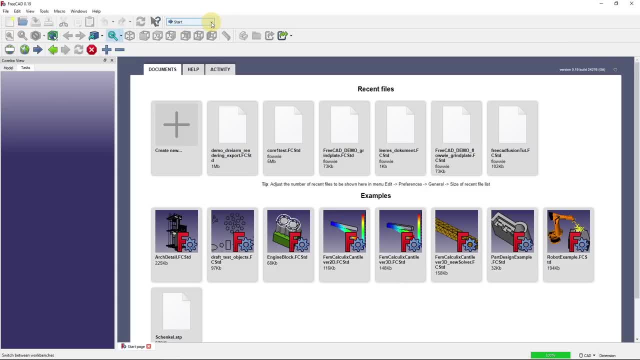 You can see that by having a look at this little button here. This is the so-called workbench selector, where you can select different workbenches for different activities within FreeCAD. What can you do in the start workbench? First, you have documents. 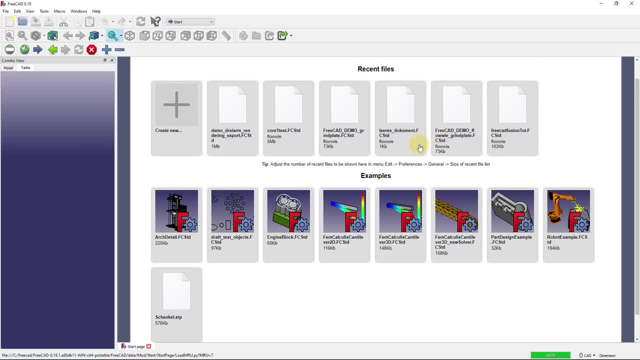 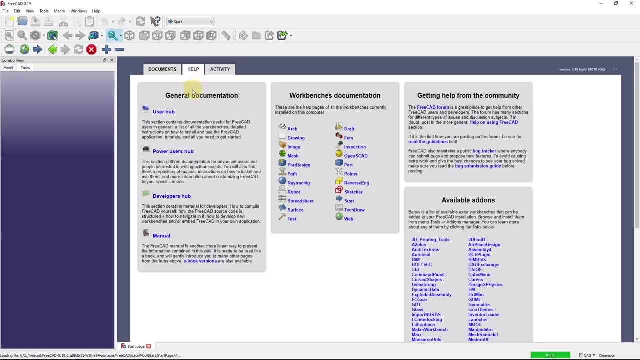 You will find the recent file list, the files that you have been recently using and some nice examples of FreeCAD. We have the help tab- very important. that brings you directly into the documentation and you will find about the different workbenches and applications you do in these. 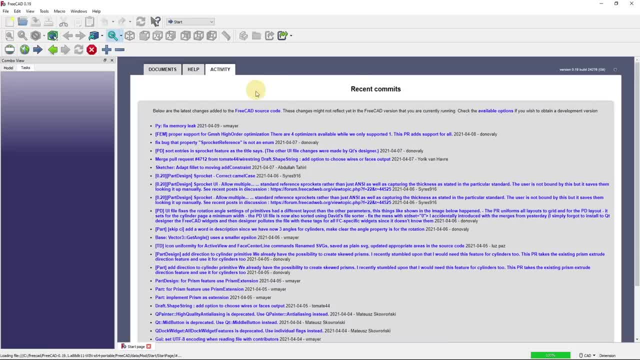 workbenches And, lastly, the activity tab. You can see the last changes that have been added to the FreeCAD source code. FreeCAD is heavily under development and you will see that there are fixes and new features coming to FreeCAD all the time. 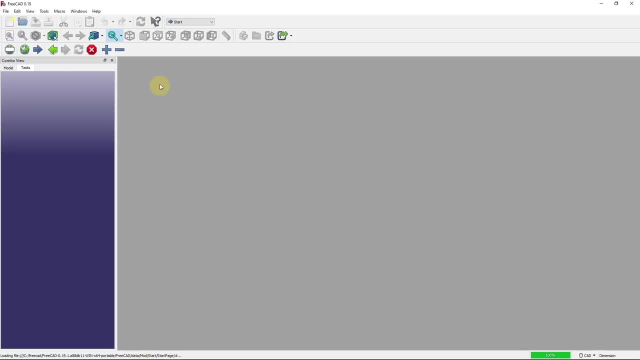 Let's close this start page, tab down here and you will see a big gray surface here. Within this gray surface, we cannot do any 3D design work. So in order to do this, we need to change the workbenches. So let's click on here. 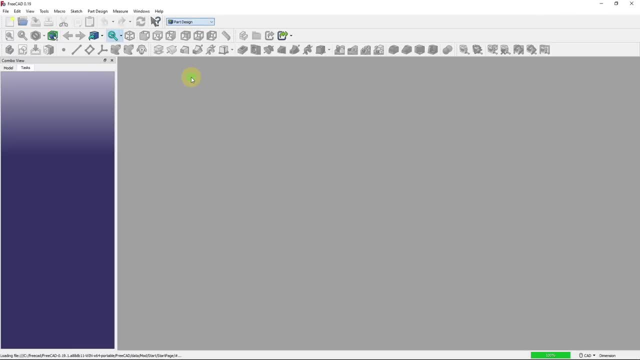 The workbench selector and select the part design workbench. Why the part design workbench? This is my standard workbench to create 3D geometry and the workbench that I will use within this course. The first thing I'd like to do is to change my user preferences. Therefore, I click on edit. 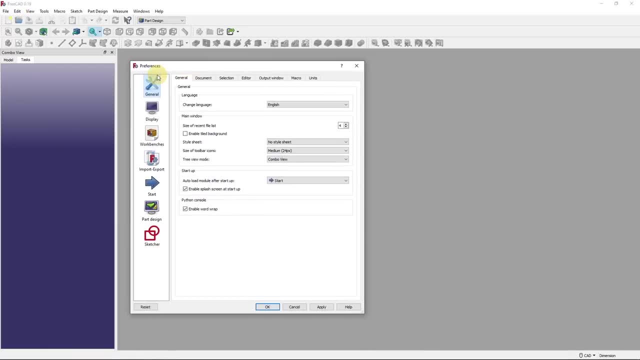 preferences and then I will have this little window here to change the user preferences. These are just suggestions By me. you don't have to follow all of these. You can take some of them. You can do it completely on your own. It's just a suggestion and it will show you how I have my user preferences set for. 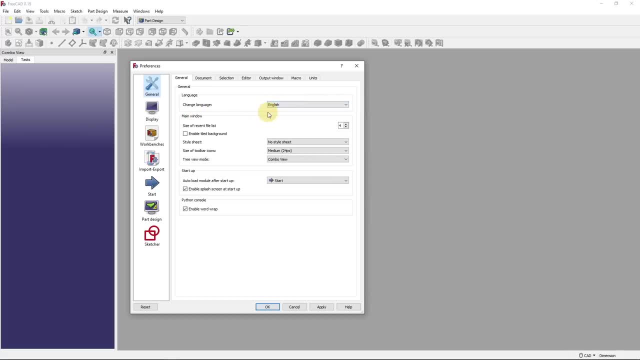 this course The language we will leave on English. First thing we need to change is the size of the toolbar icons. That's currently set to medium. These are the toolbar icons here on the top of the screen and I find them too tiny to be easily visible, So I change them to large. 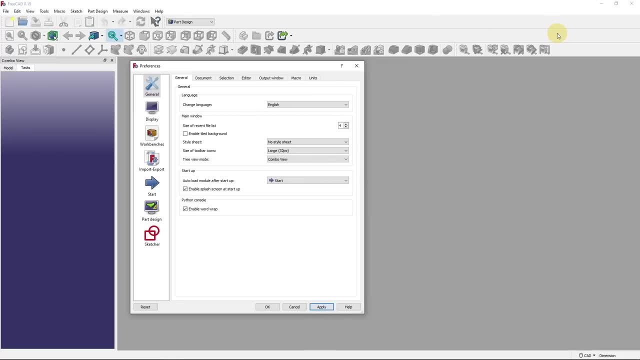 32 pixels apply and you will see it's a lot better visible. Next thing I want to change is which module is automatically loaded after the boot up. At the moment, we start in the start workbench, as you have seen. I will change this to the part design. 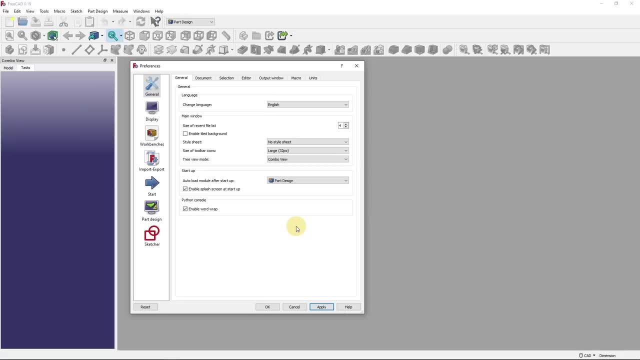 workbench and click on apply. So whenever I boot FreeCAD for the next time I will automatically start in the part design workbench. There are six more tabs under the general settings here: Document selection, editor units and so on. You can check all of these and find if there are settings that 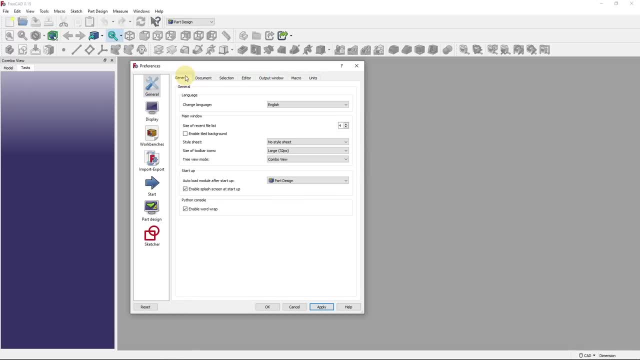 you would like to change. I will leave them at standard for this course. Next thing we click on the display, We will add anti-aliasing. That's currently set to none. We will change this to msaa four times and we will change the pick radius. So how sensitive does the selection? 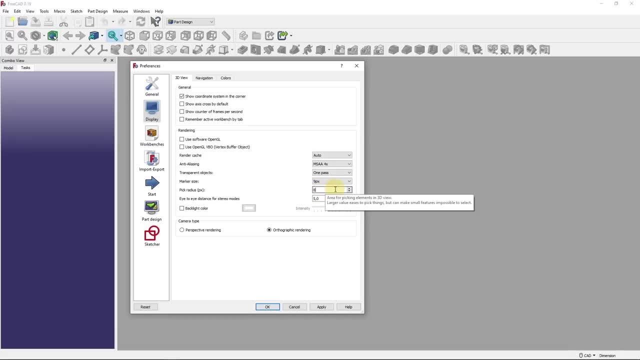 react to your mouse click. We will change this to eight pixels. Apply Under the navigation tab. we will leave everything as it's set standard. We will leave the 3d navigation at CAD style. And the next tab is important, It's the colors tab. 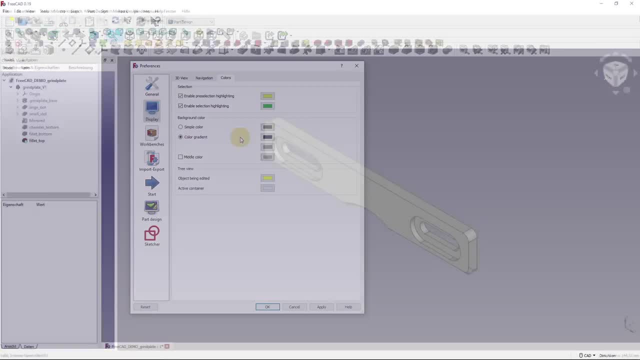 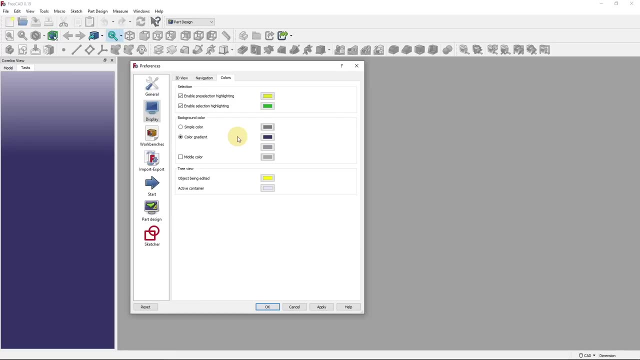 Where we have a gradient color as standard background color. You see this nice blue to gray background color. I prefer not to have gradient in my background, especially not when recording video. This can produce some unwanted artifacts by compression settings in the video, So I prefer to use a simple color. I click on simple color and change this simple color. 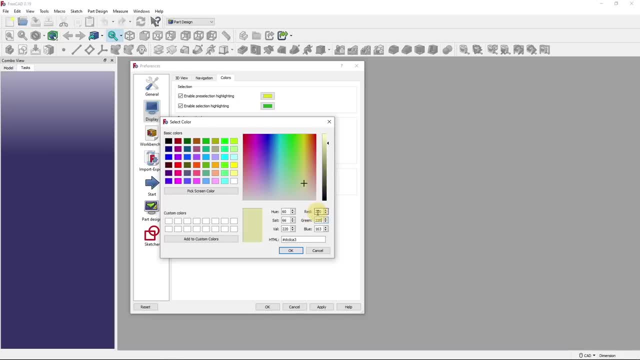 in the red, green and blue settings to 220 each. Therefore I will have a nice light gray background. The pre-selection and selection highlighting at yellow and green I will leave at the standard settings. So the next thing I want to do, I want to go to part design and change the model settings. 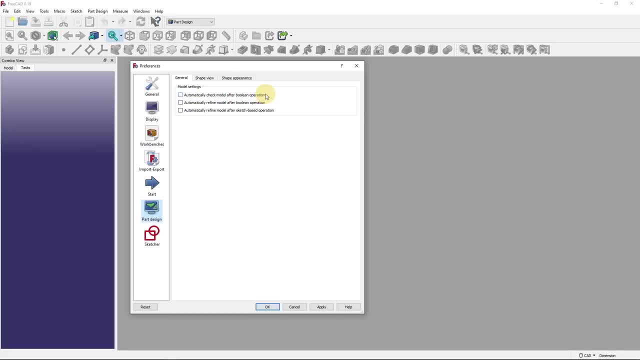 Checkboxes here to automatically check the model after boolean operations, to refine after boolean operations and to refine after sketch based operations. I will set this active, All three of them. Next tab is the shape view tab. I will change the angular deflection. 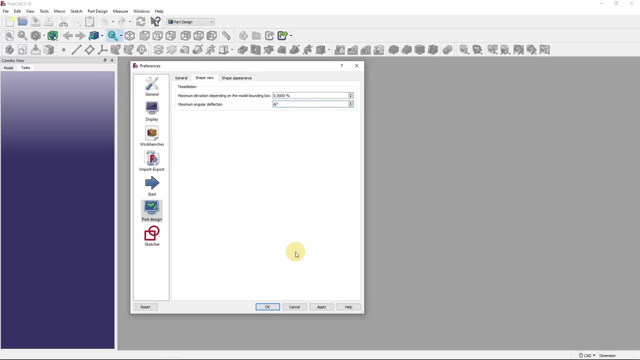 from 28.5 to 6 degrees. That means that, for instance, on a cylinder where you have round shapes will be displayed a little bit more like a round shape, but not so edgy. So I will change it to 6. Apply shape appearance. I will have to change the shape color. 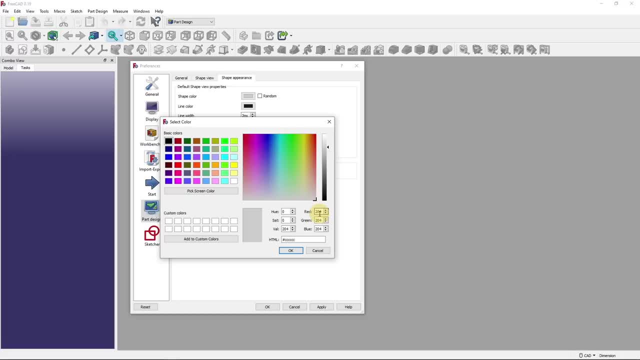 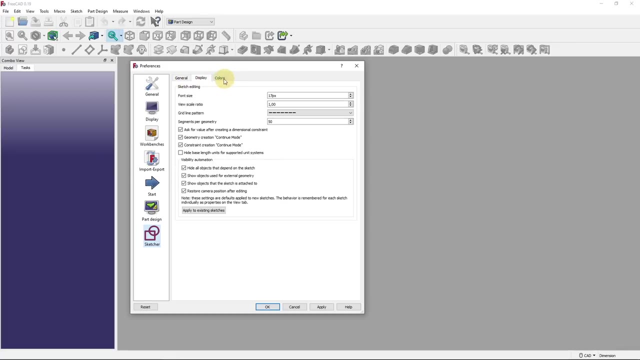 That's also set to a very light gray. This will not be visible very well, So I will change it to a darker gray. 98 each and apply. Let's go to the sketcher In general and in display tab, everything can stay at standard settings, but under colors you will see that there are a lot of different color. 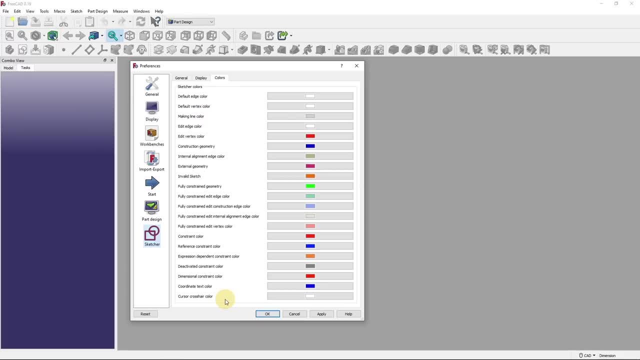 settings to be made. If you want to change the shape color, you can do that by clicking on the option in the sketch tab. Now my suggestion: if you leave the background color under display here, if you leave this at the standard setting- dark blue to dark gray background, everything with the 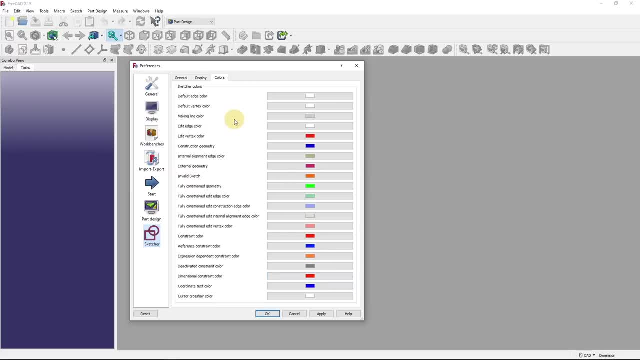 colors in sketcher is also fine. But if you change it according to my suggestion to a light gray background, you will have problems, for example, to see the default edge color at white or default vertex color at white in front of the light gray background. So you can change the shape color if you. 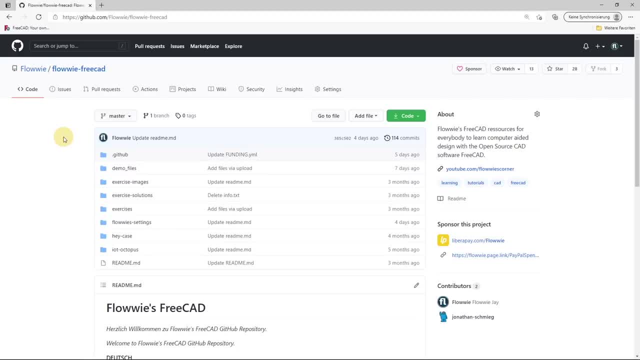 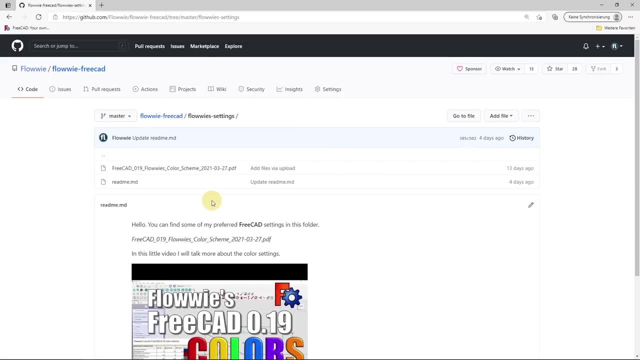 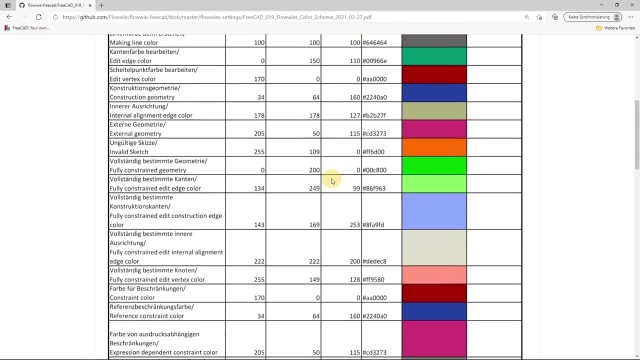 want to. At my github repository, githubcom. flowy, slash, flowy, freecat, you will find a folder flowy's settings and under this folder you will see my color scheme. That's a pdf file where I have listed all the settings for all the colors in the sketcher and in freecat in general. Maybe this can. 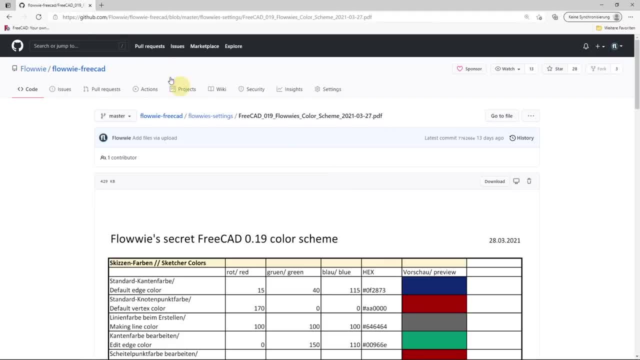 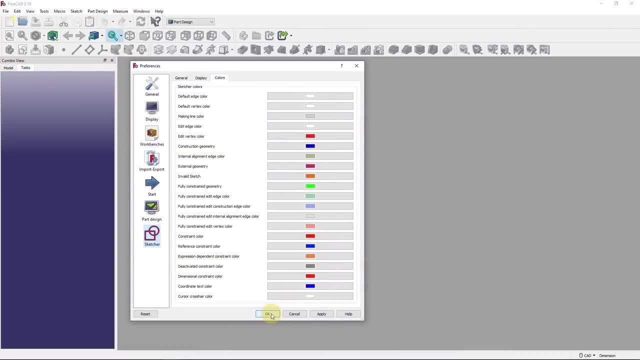 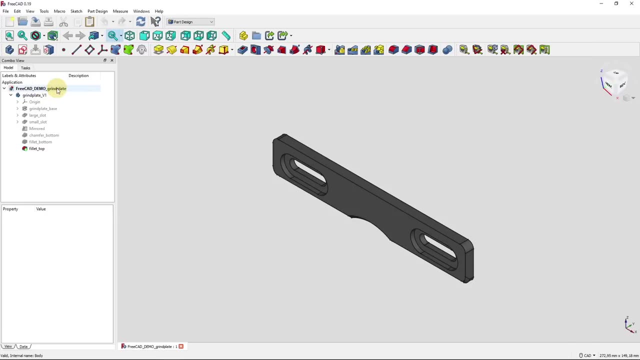 help you, and I've also made a separate video on the topic of the colors, So I will change the colors here now, and then we start in freecat and talk about the user interface. To explain the freecat user interface, I downloaded the freecat demo right blade here, also from my github repository. 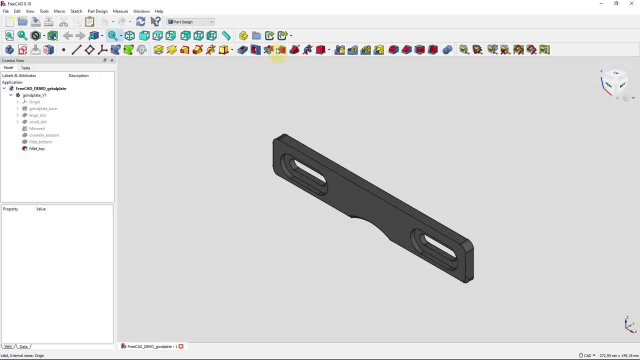 from the example files, because it's easier to explain the interface if you open a freecat file and don't show it in an empty freecat document. The first thing I'd like to talk about are the toolbars. The toolbars are located here on the top of the screen and you can drag and drop them. 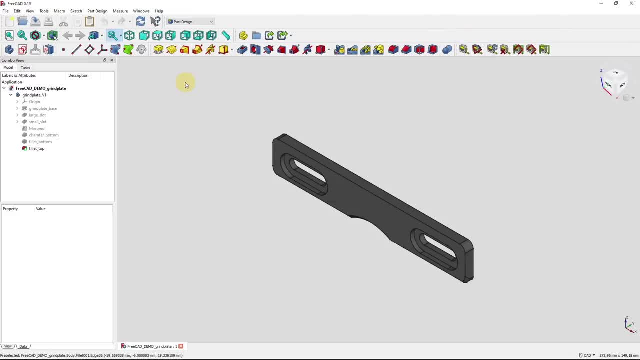 and you can also drag and drop them to the top of the screen, So you can drag and drop them and position them according to your needs. If you are missing one of the toolbars that you need, you can go to view toolbars and here you find all the toolbars that are necessary, For example, 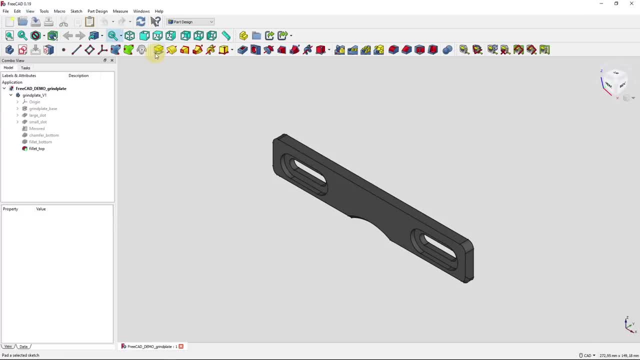 the part design modeling tools. These are the most important tools here in the part design workbench in order to create geometry. The largest part of the screen here is the 3d view, where you will see the grind plate or the 3d geometry. 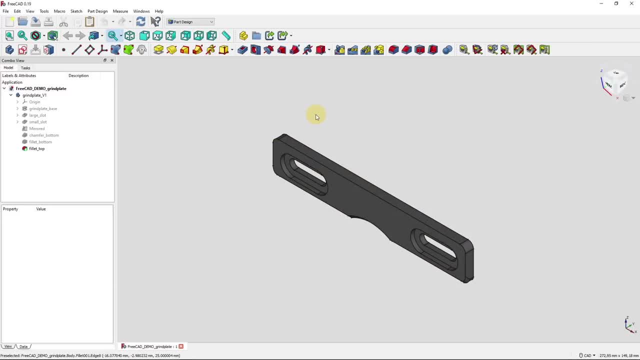 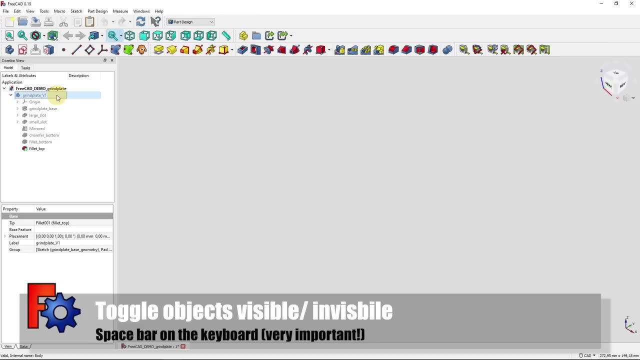 Everything that's visible here in the 3d view can be toggled visible or invisible. For example, you will see on the left side you would see the grind plate here. If you select it and you press the spacebar it will disappear in the 3d view, Press spacebar again and it's back visible. 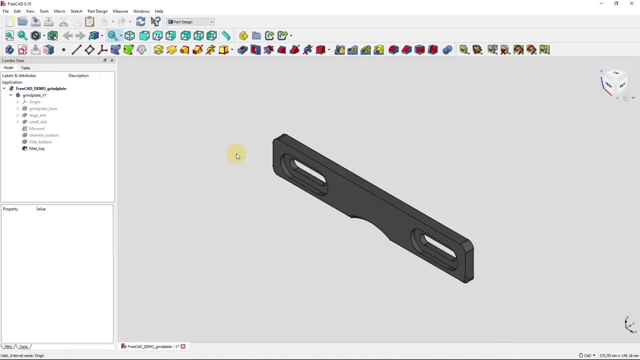 That's a common mistake among beginners: that they lose their geometry and it's simply hidden. If we hover the mouse over the geometry, you will see the grind plate. If we hover the mouse over the geometry, you will see the grind plate. If we hover the mouse over the geometry, you will see the grind plate. 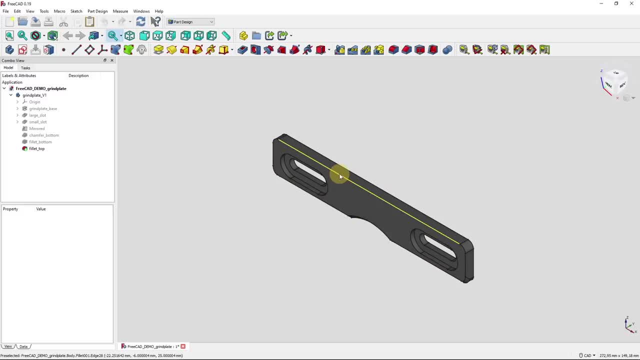 If we hover the mouse over the geometry, you will see that certain parts of the geometry, like faces or lines, are yellow. That's the pre-selection color and if you left click on it you will see it turn green. That's your selection color that you can set up If you want to select more than one. 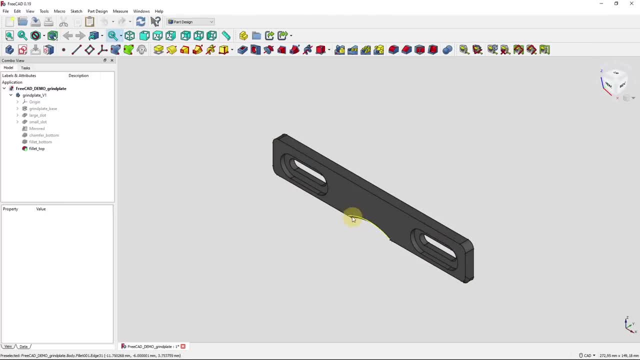 object. you will have to hold down the control key on the keyboard and select more elements, For example these four faces. If you click the empty screen, everything will be deselected. The controls in the 3d view are defined here on the bottom right of the screen. 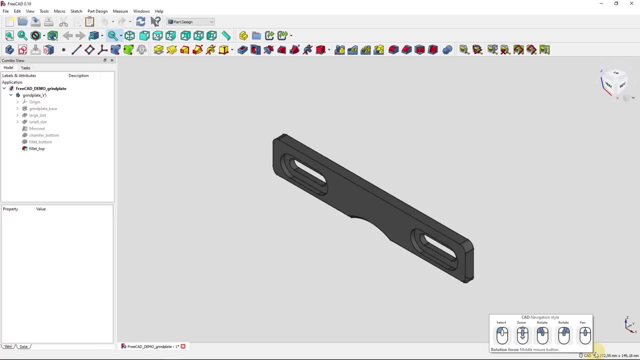 If you hover over it, you will see that we have the cat navigation style that we set up under the settings. It's selecting its left mouse button, zooming is the mouse wheel, rotating is middle and left or middle and right mouse button, and to pan we press the middle mouse button. So we start. 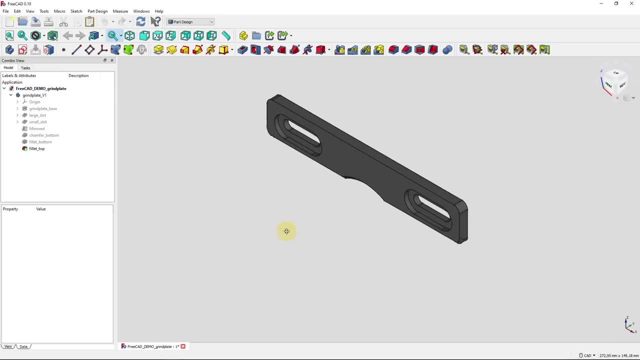 panning. I press the middle mouse button and I can't pan my own 3d view. I can't pan my own 3d view. I can't pan my object here in the 3d view. I press middle and right mouse button at the same time. 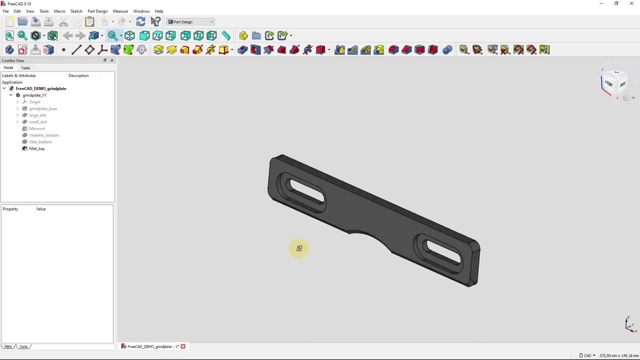 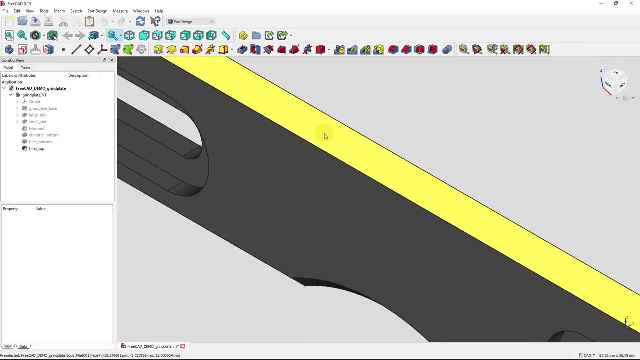 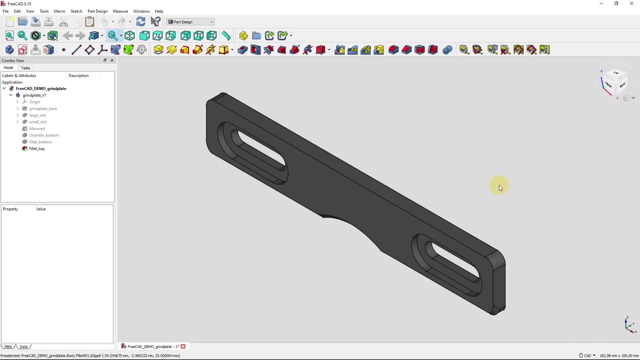 I can rotate around my object here, and if I want to zoom I just roll the mouse wheel back and forth, and so I zoom to certain elements. The focus point on the zoom is always defined by the location of your cursor. If you're completely losing track in the 3d window, 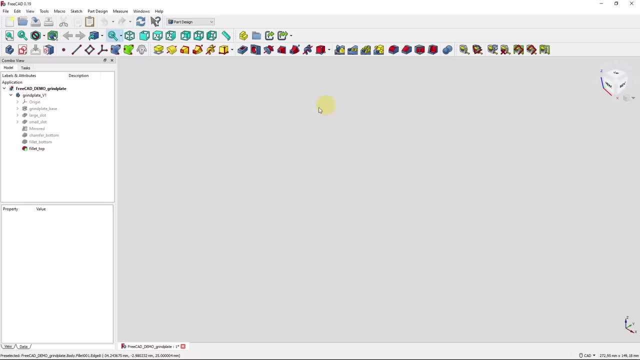 what can happen pretty easily, for example, if you pan it out of sight. here there is help for you. In the top left of the screen is here the button. fit the whole content on the screen and you will see the part appears back in the middle of the. 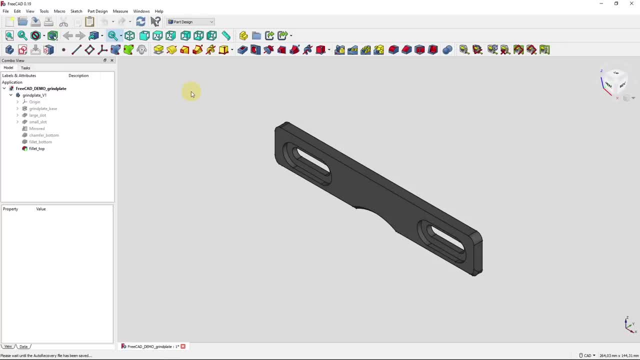 screen, So always remember this button here. What I often do is, when I'm constructing, I use these predefined views. here We have the isometric view that we are currently in. we have a front view, a top view, view from the right side, view from behind. 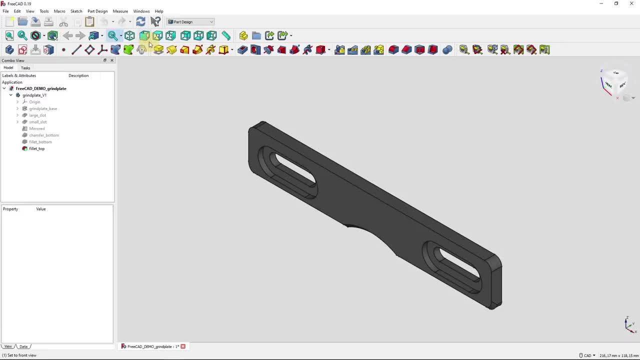 down and from the left side. These are very helpful and I often use them. We also have the navigation cube on the right corner of the screen where we can also select various angles of the geometry, and I often use the cube to keep track in my 3d orientation. 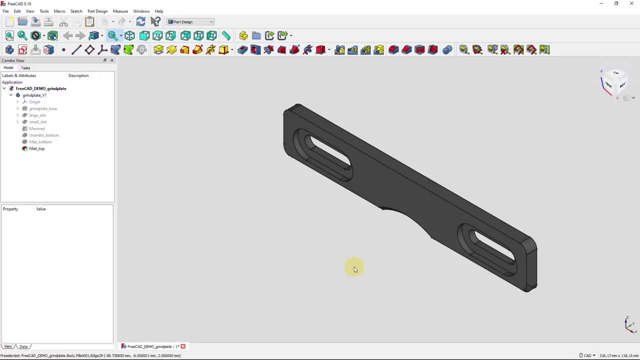 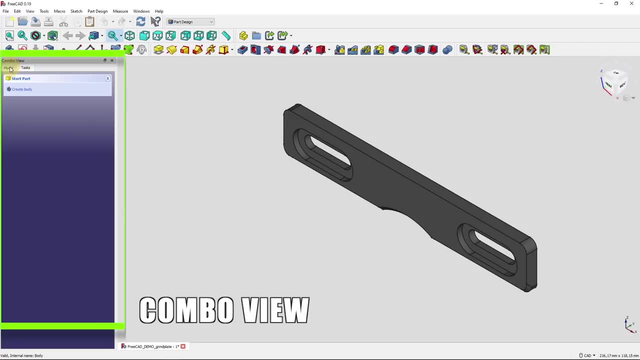 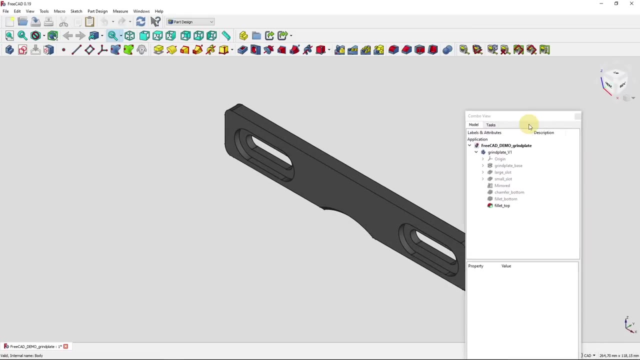 And the last very important thing in the FreeCAD user interface on the left side of the screen is the so-called combo view. that's divided under model and tasks tab. here. The combo view can also be grabbed here and positioned on a different place of the screen. 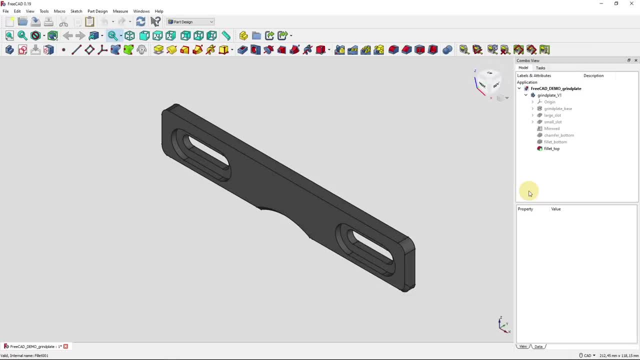 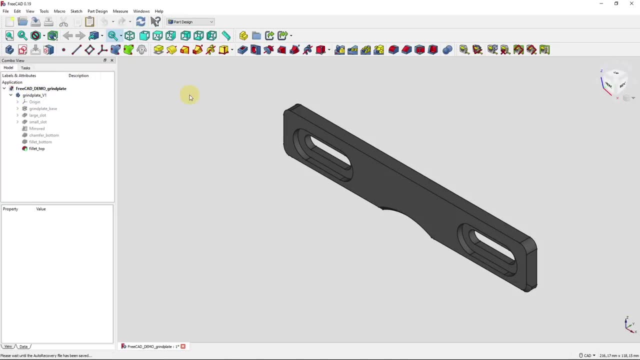 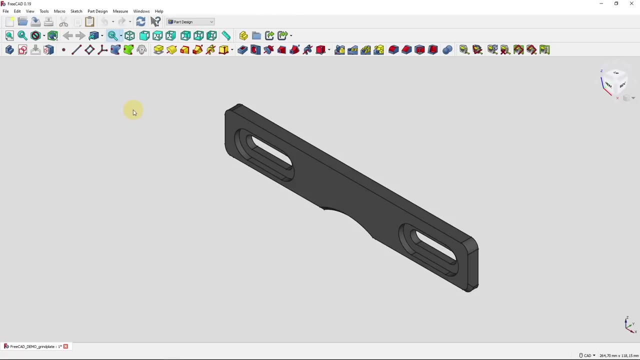 for example, on the right side, which is standard in some other 3d CAD programs. I leave it on the left side, but you can drag and drop it where you want. Something that can also happen is you click the little x here on the top right and you click close, and now you don't have the combo view anymore. 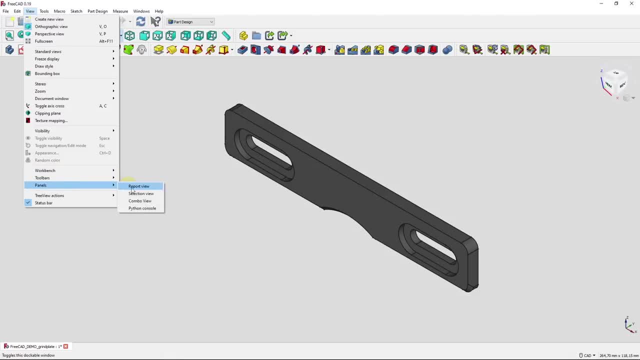 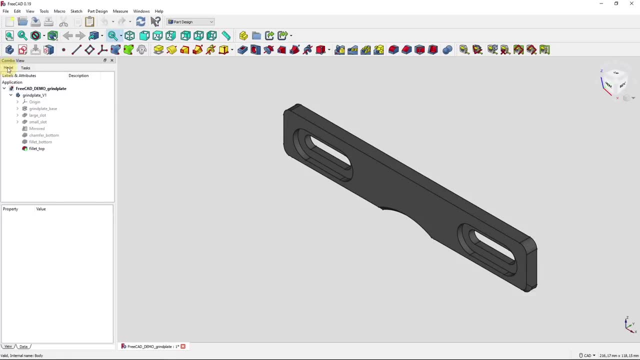 You have to go to view panels, combo view, to make it appear again. You should not close this. it's very important. Under the model tab in the combo view you see the model tree. So how is the 3d file you see here in? 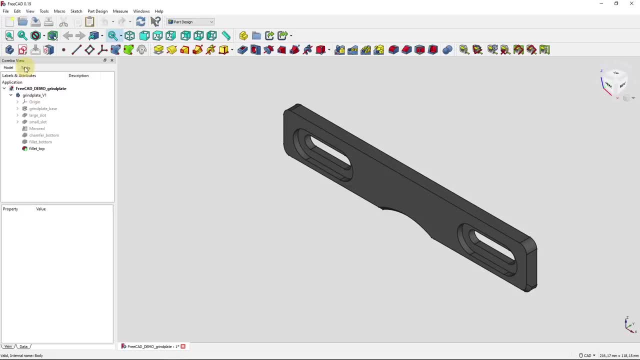 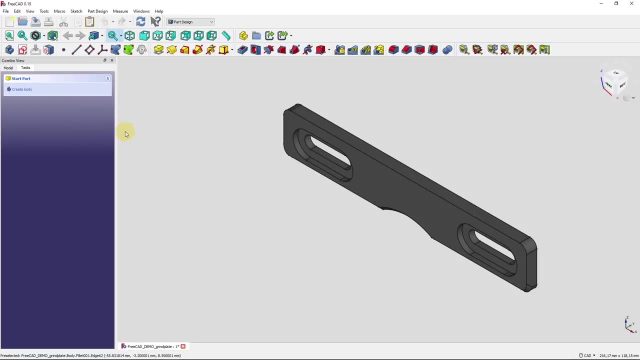 the 3d view. How is it structured, And under the tasks tab you can do various operations. These operations depend on what you have selected. For example, if I select this edge here, on top of it, the tasks tab will change to give me the option to. 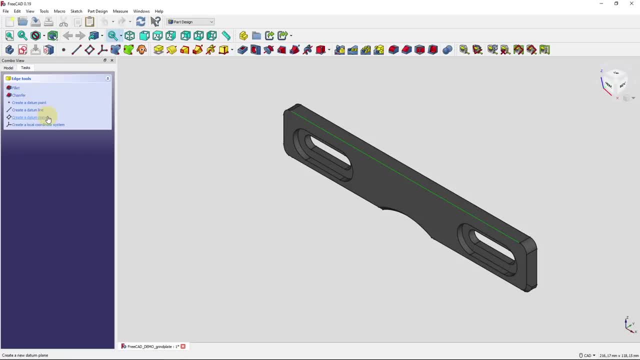 create a fillet or a chamfer here or some datum geometry so I can select chamfer and create a chamfer here on the edge. So it's sensitive to what you have selected. If I have nothing selected, like now, the tasks tab offers me to create a complete new. 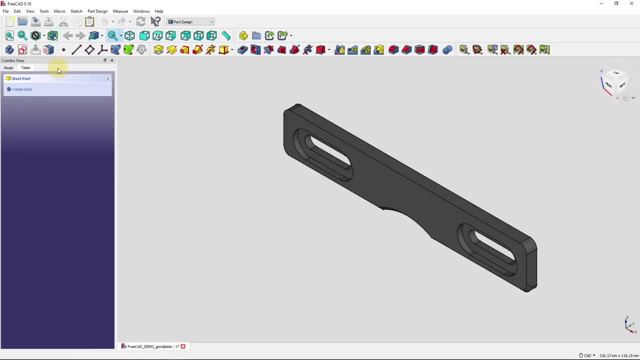 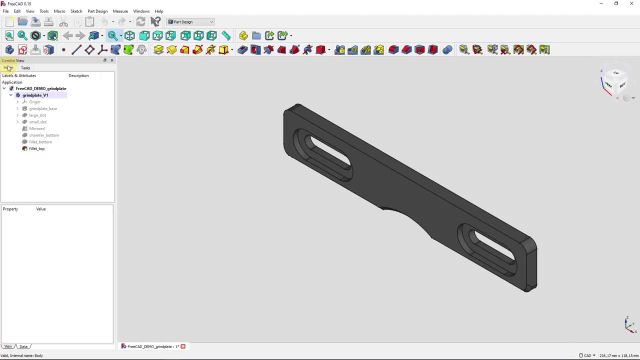 3d body element. You can simply switch back and forth between model and tasks tab by simply clicking on it. As I said earlier, model tab: in the combo view you'll find the structure or the composition of your 3d file. let's have a closer look at it. the first thing is the actual file. if you select it, you will find. 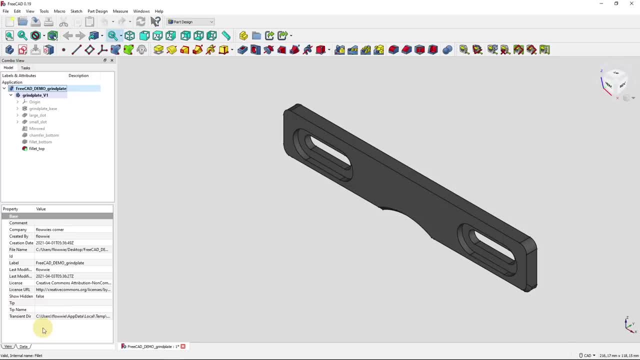 different informations down here under the properties about the file. so, for example, who is the creator of the file, where is it located on your hard drive and other things like license and other informations about the actual file. the next thing is the part design body. it's called. 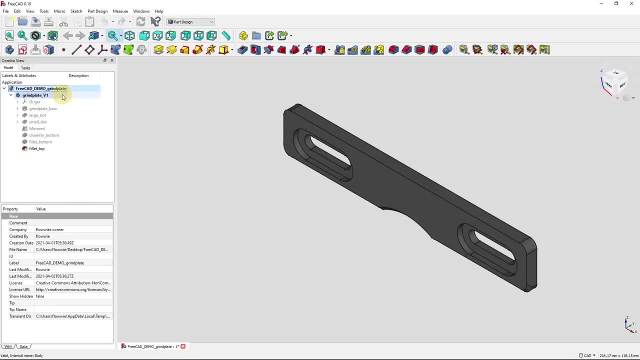 grind plate. underscore v1. in my example here, if i select this, a body element is very important in the part design workbench because under the body element it's like a container. all the 3d and 2d geometry belonging to this will be stored in this container. for example, all the sketches, all the 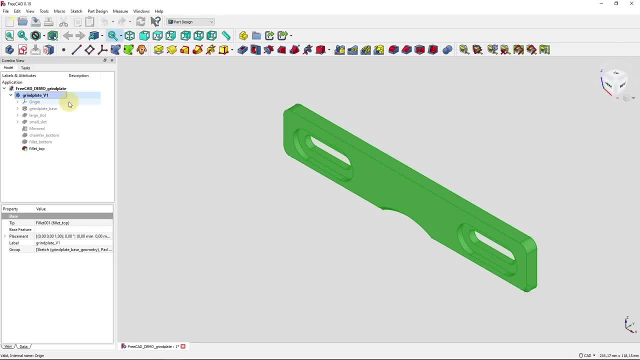 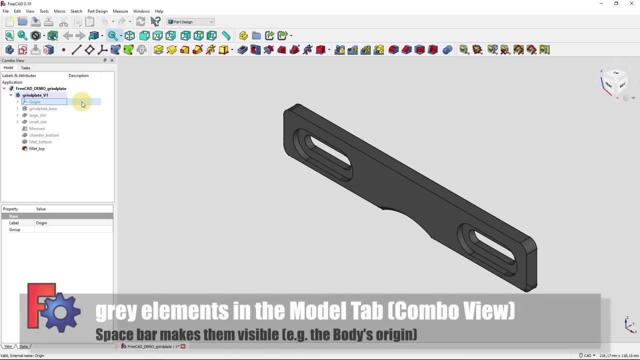 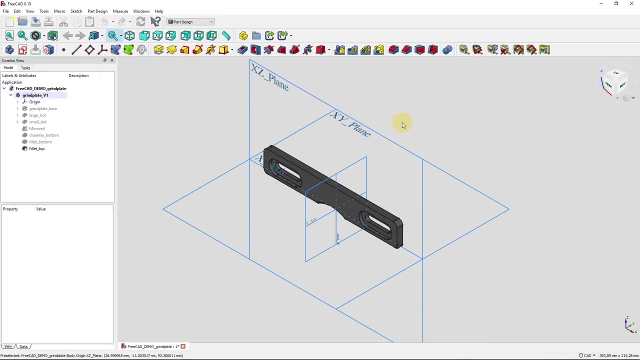 operations features. every body has its own origin, and that's the first thing you find in the list. under the body here, origin, it's grayed out, so we press the spacebar and make it visible. you will see then that the origin consists of three planes: x, y, xz and yx plane and three x's. there is a little arrow next to origin. if we click on that. 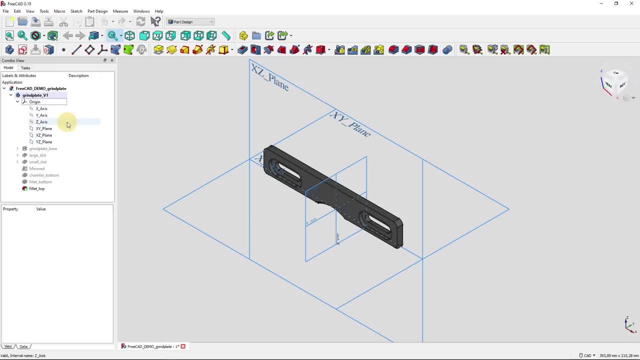 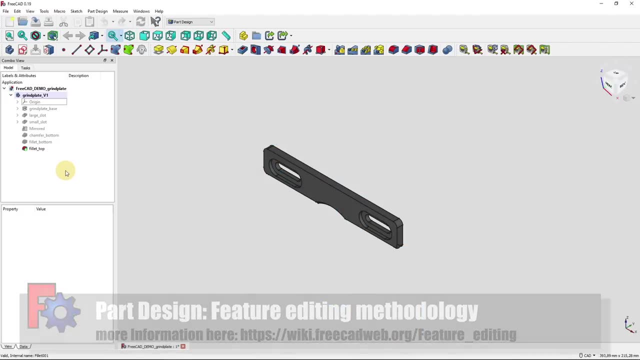 you will see that there are the six elements that make the origin in part design we talk about, based on Lucy Farc's example. i will click here and then we're going to show you what we're so-called feature editing approach. that means that we start with one base feature and apply. 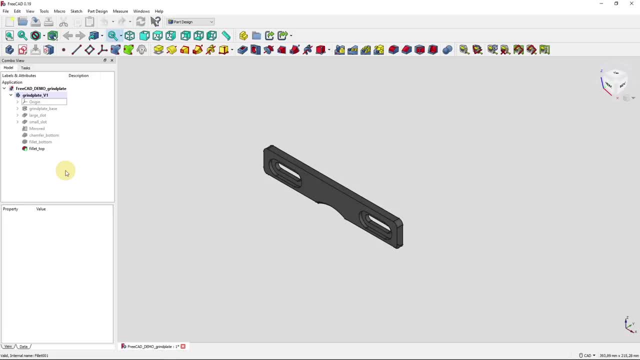 various features or operations on this base feature in order to create our 3d geometry. for example, in the model tab you see that all objects are grayed out, only fillet underscore top is in color and that means that only the last feature here is displayed. we can select an earlier. 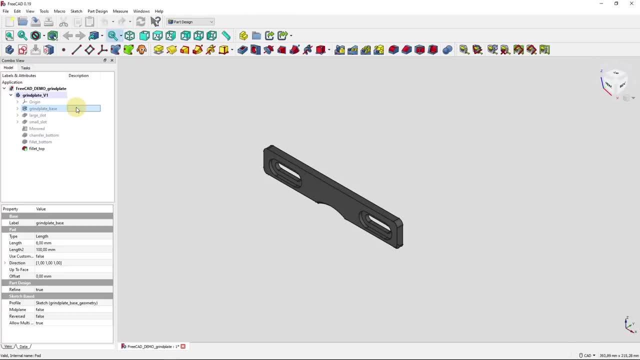 feature, for example, the grind plate base. press the spacebar. you will see that fillet top will become grayed out and we only have grind plate base colored here. this is almost like jumping back in time to the timestamp when this feature was created. how was the grind plate base created? 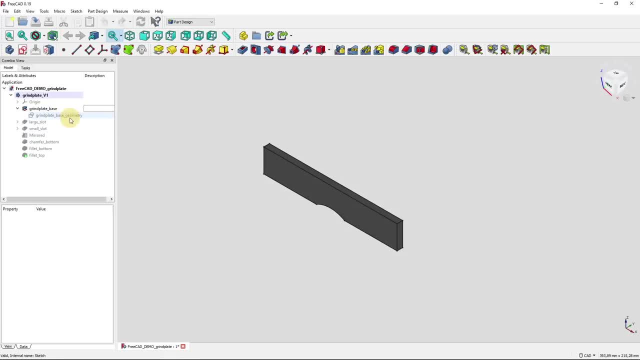 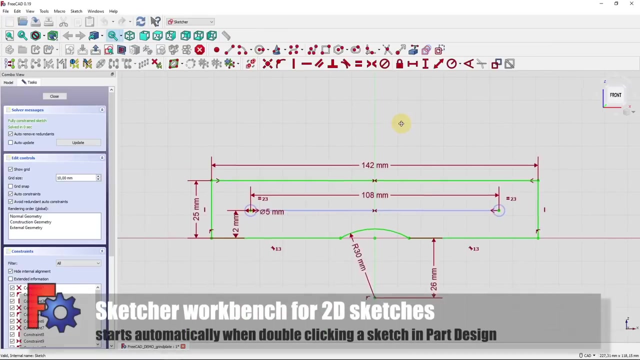 we click on this little arrow and we see an underlying feature here called grind plate base geometry. with this little icon here we can also make this visible by pressing spacebar. and on the back of the geometry we will see some lines here, these blue lines and red dots. i double click on this one and you will see. 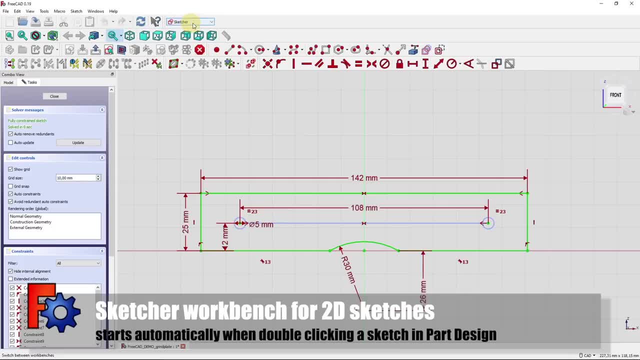 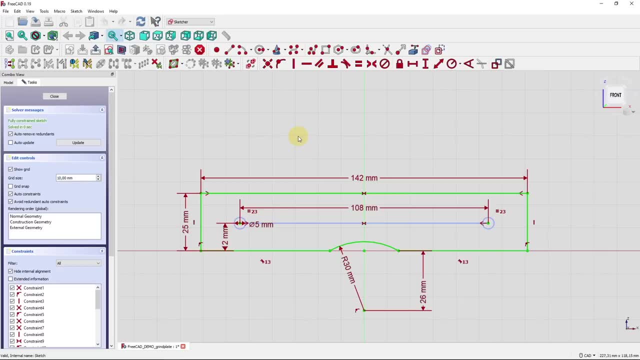 we move to a different workbench, the so-called sketcher workbench. that's a 2d workbench where you can define two-dimensional sketches to define your geometry. i close the sketcher and this sketch was modeled to the point that the guide is shown here. you can see that the skeeecher 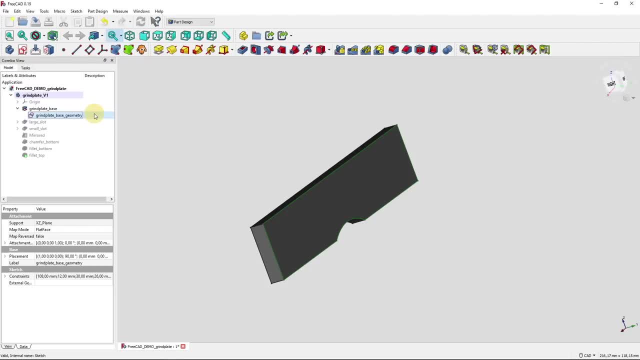 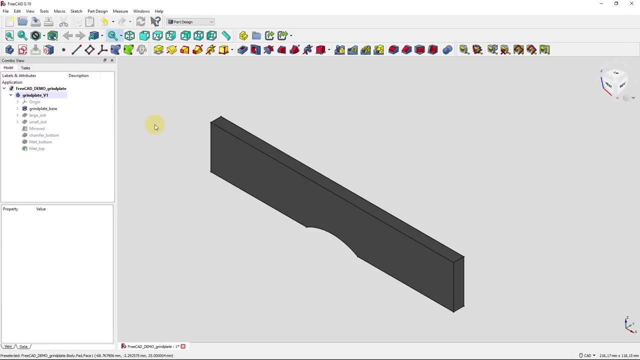 is on the right side of the sketch, and now we can move to the left side of the sketch, where I can, losing the pad to transform a two-dimensional sketch into a three-dimensional body, and that's exactly what the grind plate base here is. so now let's see what history based operation means. I created a large slot. 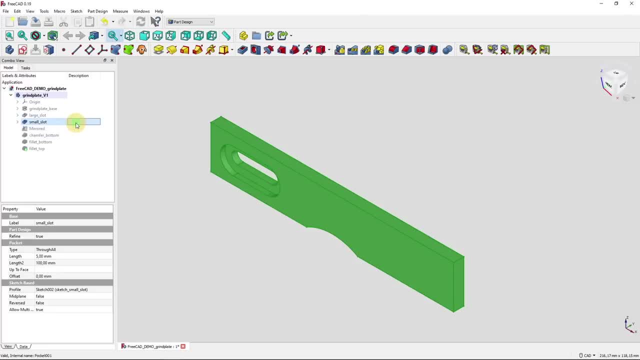 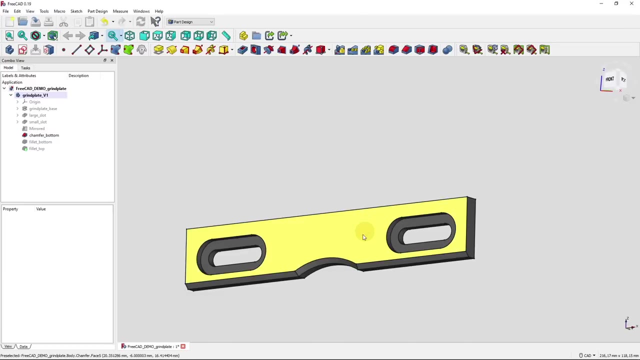 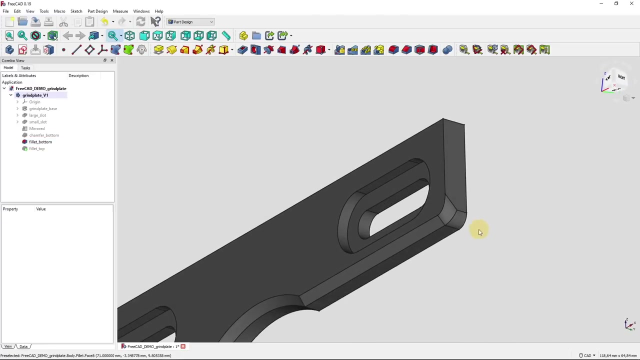 also with an underlying sketch. I created this small slot here that creates a hole in the geometry. I created a mirror that mirrored the two slots here. to the right side I created a chamfer to make a little chamfer on the down edge here. then I created a fillet that rounded the corners here and then I created another. 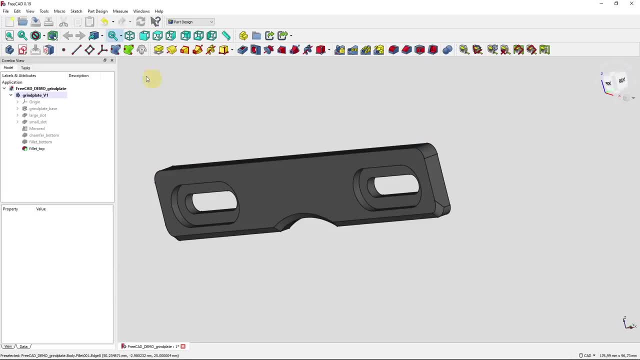 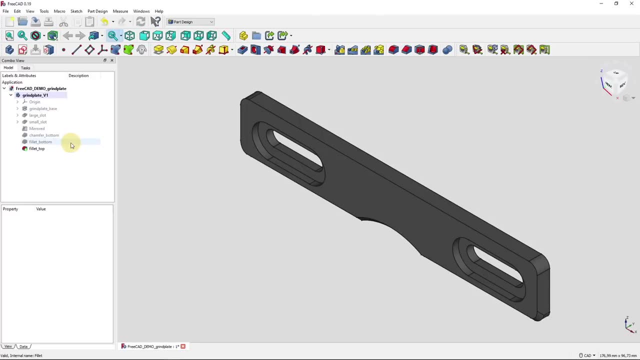 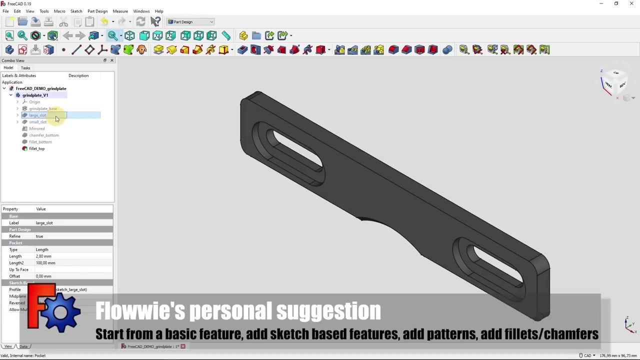 fillet to round the upper corners here. and that's the editing history. you see that I apply feature after feature to create from a simple base geometry the finished product. and what you can also see is that I started with sketch based operations like this: grind plate base that's a pad and the pocket for the slot holds here and after. 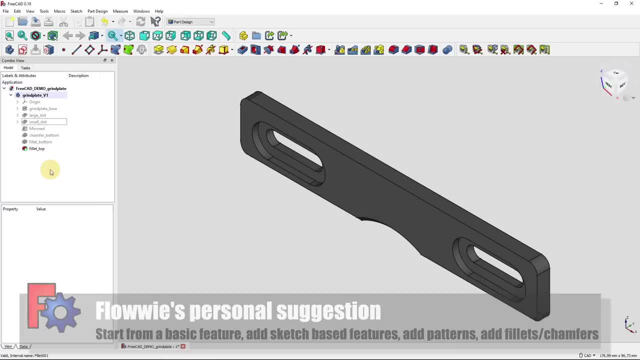 I was finished with the sketch based operations, then I moved on and created features that lay on top of 3d geometry. for example, the fillets here are not based on sketches, they are based on 3d geometry and it's always advised to use these elements that are based on 3d 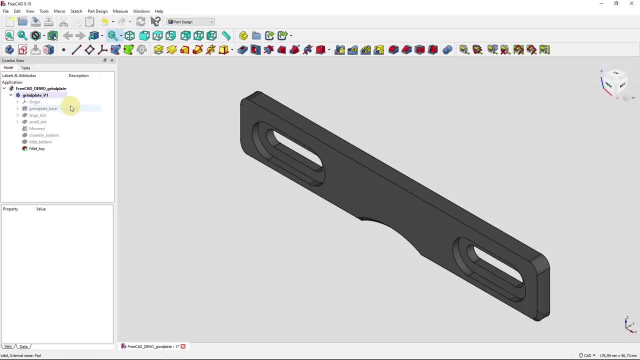 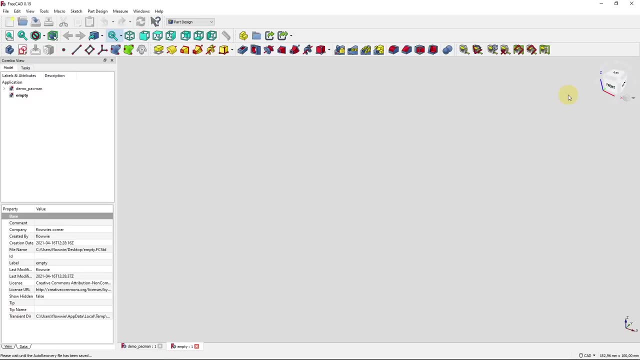 geometry as the last elements in your structure. here in this part of the video, it's time to create our first very own model. I want to demonstrate two different ways to create our first model in free cat. what you want to do together now is to create this little pac-man shaped model. it's a very, very 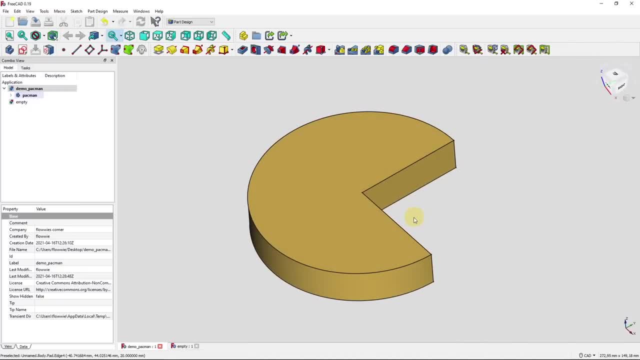 simple model. it's only a cylinder with one quarter cut out, so super simple, super easy for any one of you who has never used free cat before. first I'd like to show you how to make this model using basic shapes, and then I want to show you how you can make this model using 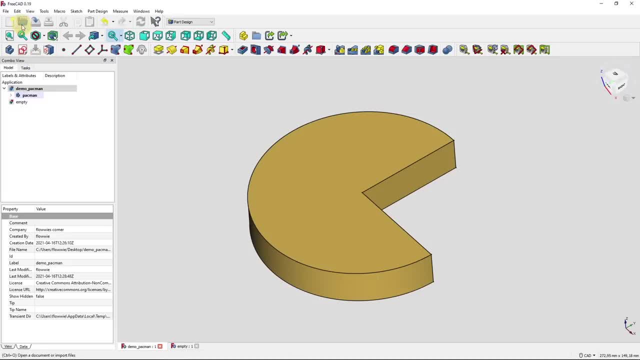 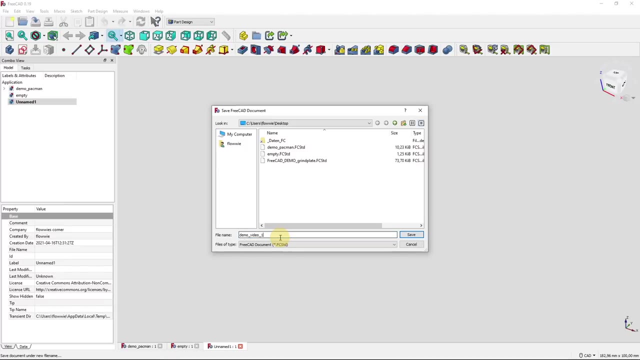 sketches and a pad. the first thing we need to do is to create a new file. we go to file new and there it's called unnamed one. we go to the safe command, save the active document, demo video one. and we have to make sure we are in the part design environment if we 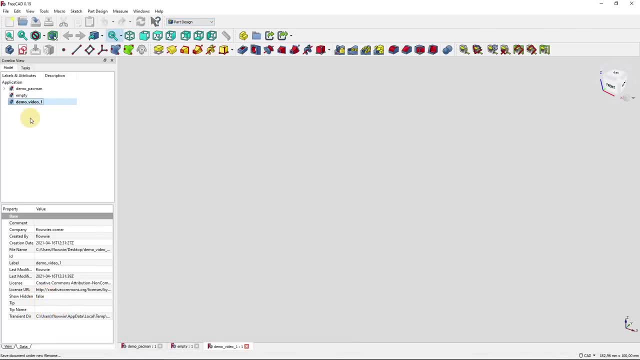 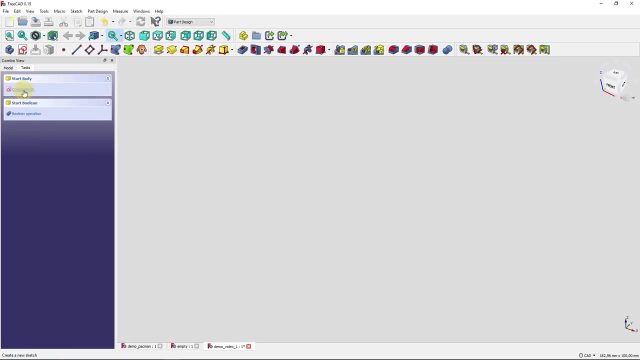 are in the part design workbench. we can create a new body element by clicking on this button here- create a new body and make it active, or click in the combo view under tasks, create body. these two commands are exactly the same, so I will click on create a body, switch to the model view again and there 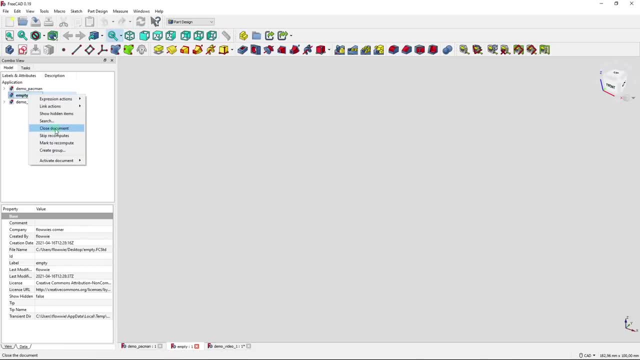 you see, I will close these two documents here and here you see the file demo video, one. that's the name of the file, and under the file there is my body. body is a container that contains, oh, my 3d and 2d geometry, and within this body, 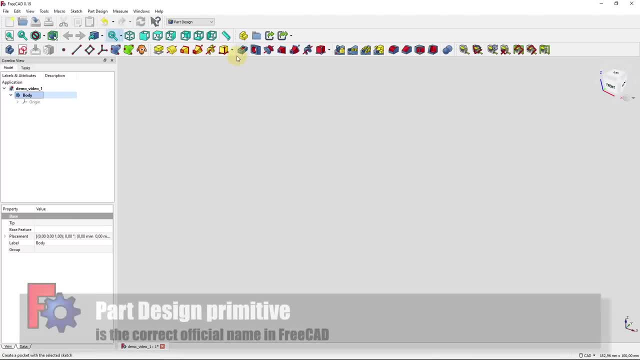 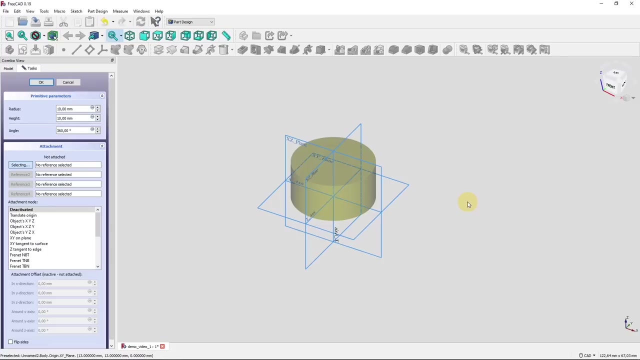 I will start doing a basic shape. therefore, I go to this comment here. primitive, that's your official name for basic shape. click on the arrow and create an additive cylinder. Now FreeCAD needs to know where we want to create the cylinder. Therefore, we need to define the attachment. 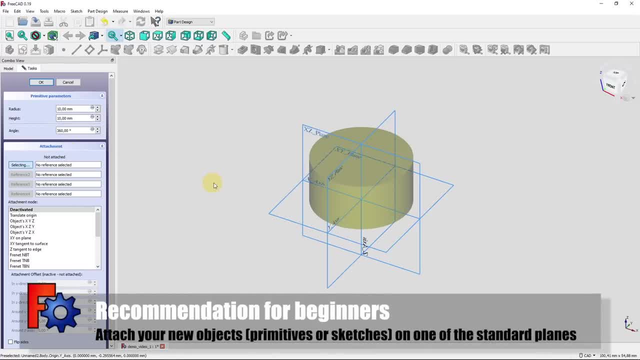 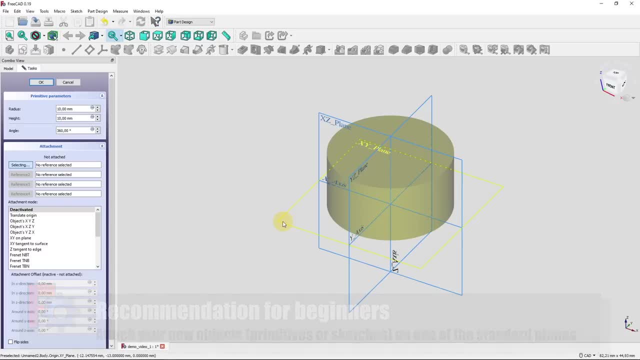 The attachment is active right now. Therefore, we can click on a plane. We have the XZ, YZ and XY plane. I will click on this plane, the XY plane, and define my cylinder to be created on top of the XY plane. 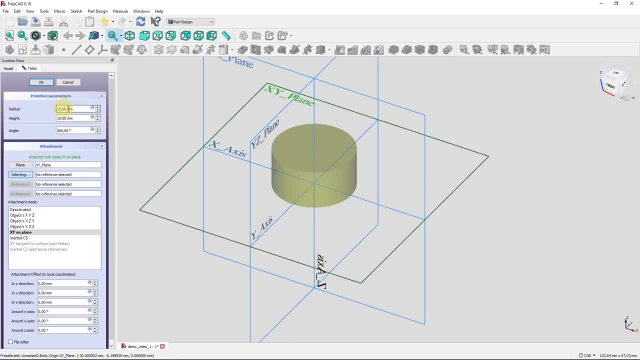 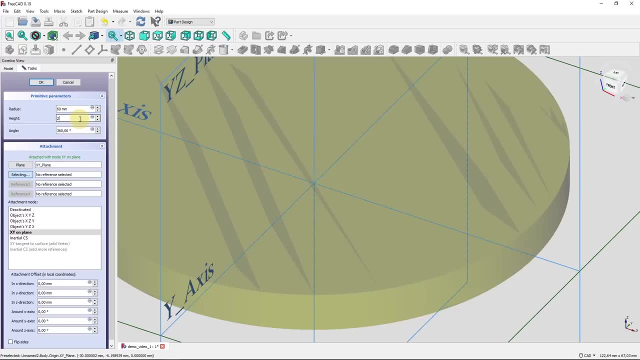 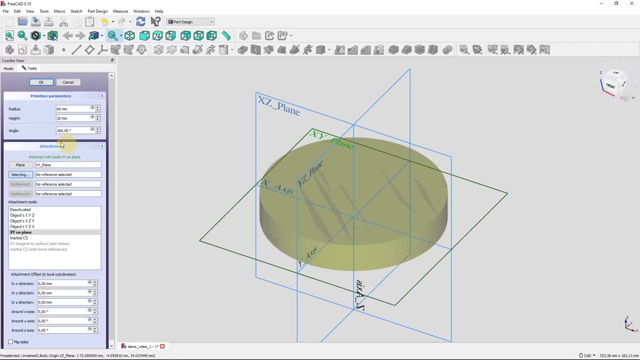 The next thing I need to do is I have to define a radius for my cylinder. I will type in here: 60 millimeters and a height of 20 millimeters, And FreeCAD is very handy here, because we can cut out the quarter by simply defining an angle here. 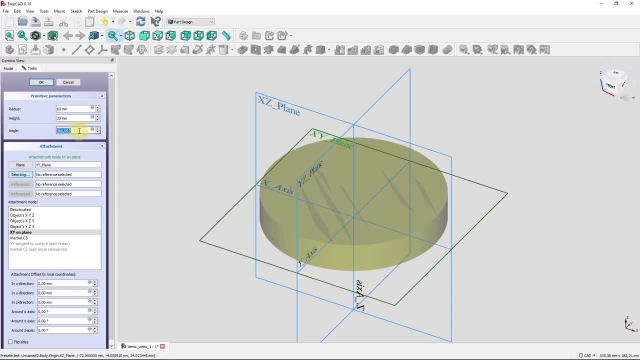 You see, it's currently set to 360 degrees. If I set it to 180 degrees, you will see I only have half of a cylinder. Therefore, I just enter 270 degrees. that's three quarter of a cylinder and I'm completely finished. 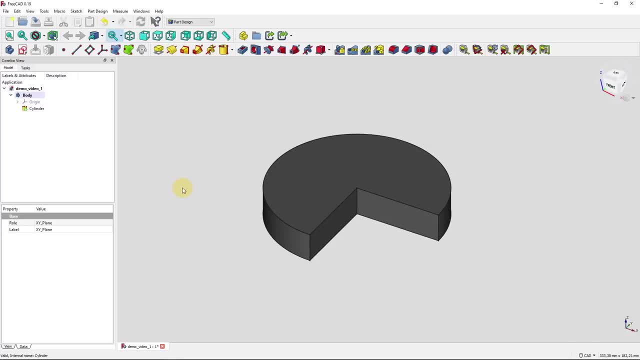 I click on OK and I have my shape completely done. I often mention that FreeCAD is a so-called parametric CAD system. That means that this cylinder is created using parameters. Therefore, I can click on the cylinder and set its properties down here. 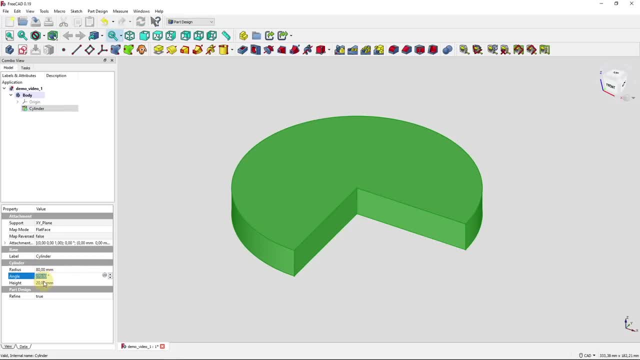 I can change the radius maybe to 80 millimeters or the height to only 5 millimeters, And the cylinder will adjust within a few seconds. So I'm set it back to 20 and 60 and can change whatever I'd like. 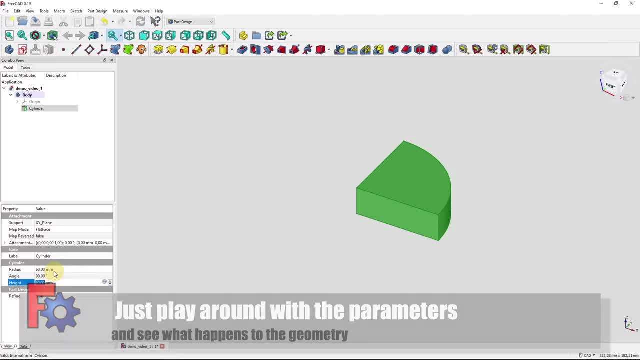 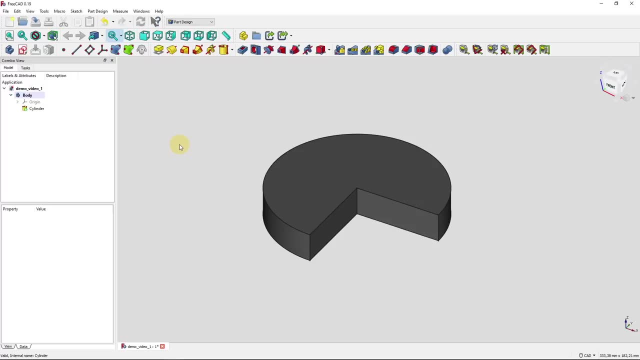 I can even change the angle here later to set it to 90 degrees. I only have one quarter. I think you get the trick. So that's when you start with primitives or basic shapes. Now I will delete the cylinder. I select it here in my combo view and press the delete button on the keyboard. 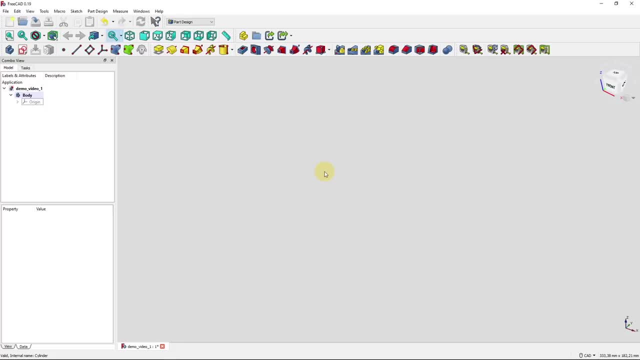 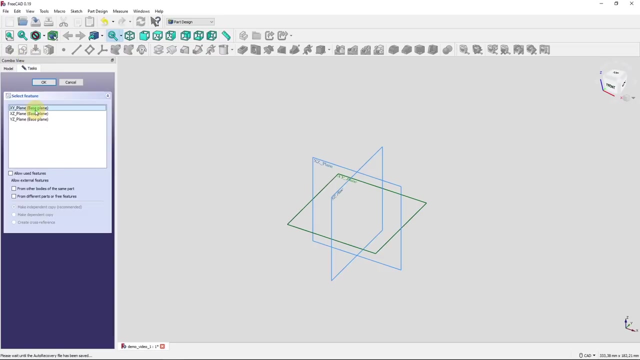 And now the cylinder is gone. The next method is using sketches. Sketches are 2D geometry that are later put into 3D space using different 3D commands. I start clicking on create a new sketch command. Select the XY plane as before, to create my sketch on this plane. 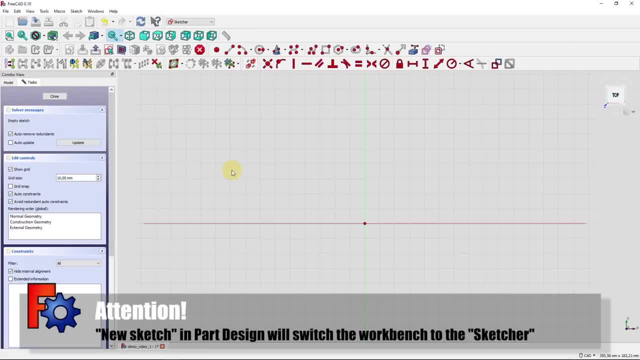 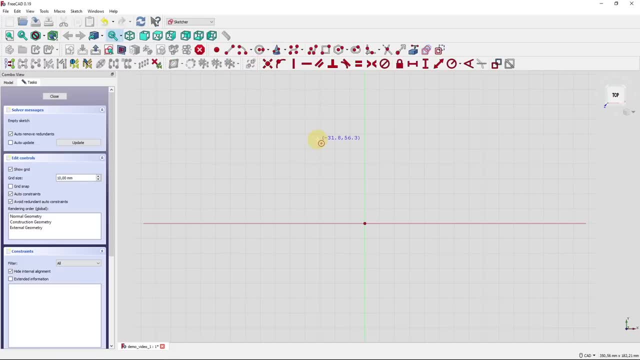 Click on OK. Then I will have to draw a circle first. I find the circle here in my sketcher toolbar. Create a circle in the sketcher. It's defined by clicking on the midpoint and one outer point. I click right in the middle of my sketch document on the origin here. 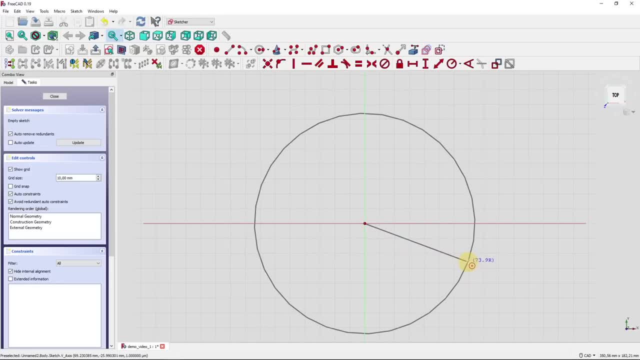 And then I drag the mouse and click again, And then I set my circle. I have to define the radius of the circle now, So therefore I click on this command here. Constrain an arc or circle. Click on the circle and set it to 60 millimeters. 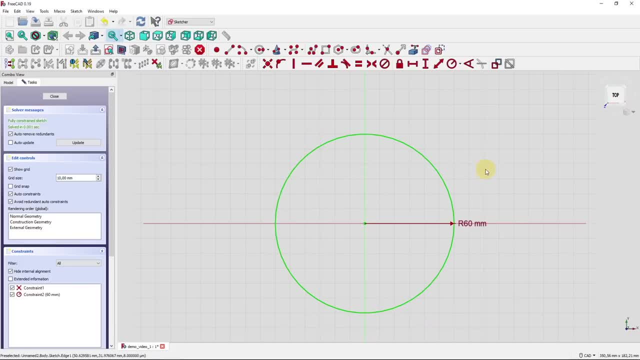 And OK, Now we have a full circle, But we only want three quarters of a circle, So I have to trim one quarter here on my circle. In order to do that, I click on the align command here: Create a line in the sketch. 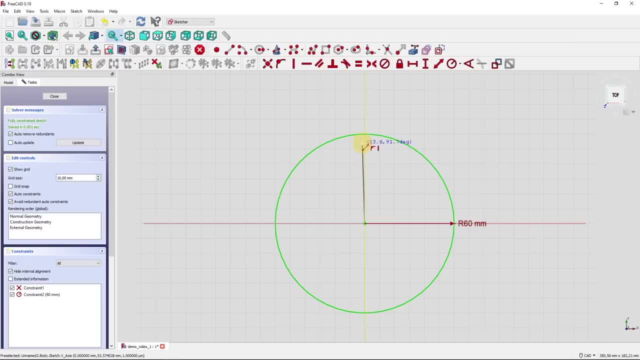 I start with the first point, also here in the origin, And I end on my circle here. And I do exactly the same starting here on my origin and end here. You will see that there are automatically two constraints created: A vertical constraint here and a horizontal constraint here. 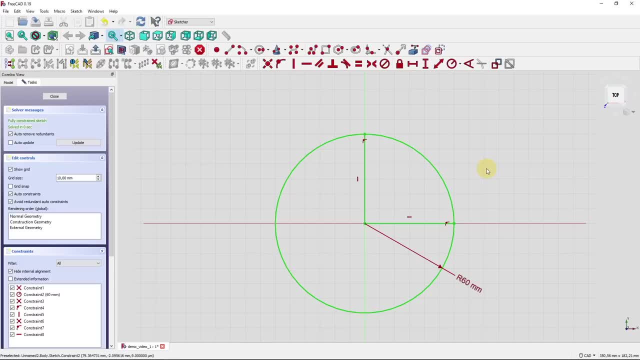 Now the sketch is a little bit over defined Because we don't have one single closed shape, but two of them. So therefore we have to trim this quarter. We select the trim command, Trim an edge, And then we click on this part of the circle. 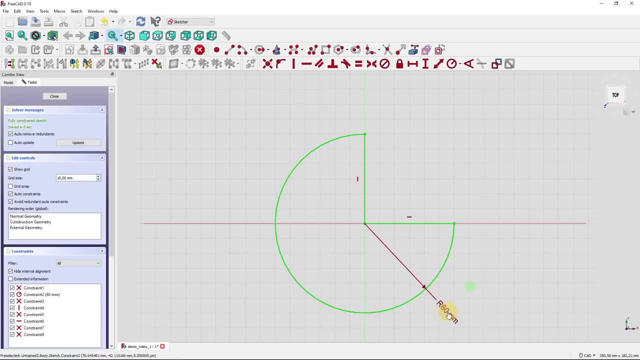 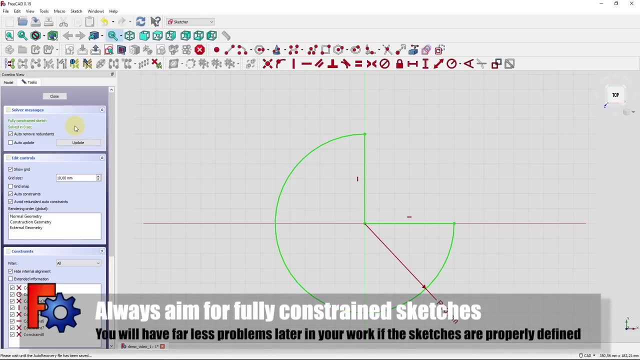 Right click to exit the command And you will see we have a three quarter circle here. That's fully constrained. You see it here in the solver messages- Fully constrained. That's what we want to achieve in the sketch. We go to close. 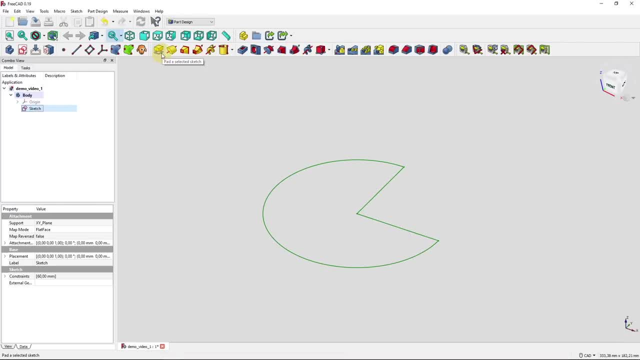 Have the sketch here, Go to pad. Pad is selected, sketch And pad it up to 20 millimeters. And now we achieve the exact same what we had with primitives before. This construction is also parametric. That means if we want to change the thickness of the cylinder, 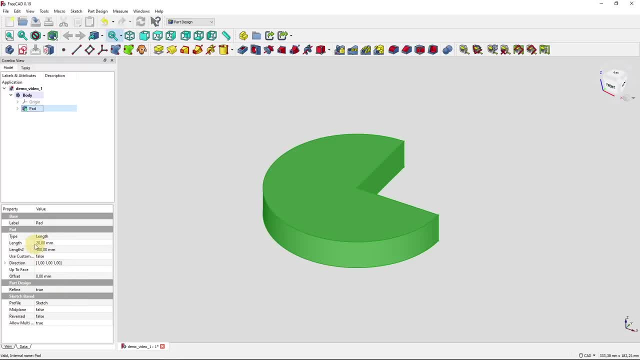 We just can go to pad And adjust under length here The height of the cylinder, Maybe 10 millimeters, 5 millimeters Or even crazy 80 millimeters. Whatever we want to do, If we want to change the shape of the circle, 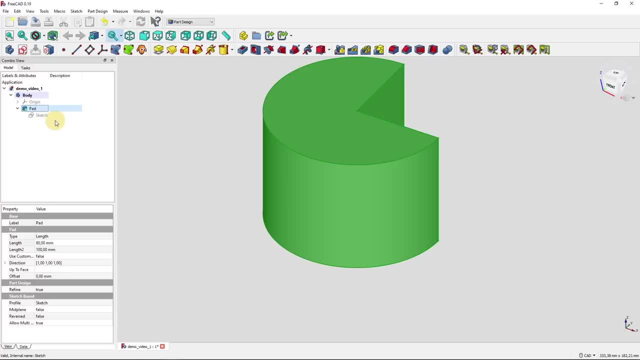 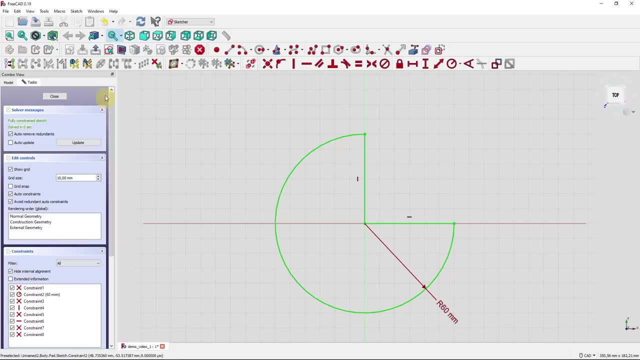 Of the underlying circle. We don't necessarily need to go into the sketch. We could do that by double clicking on the sketch And change the 60 millimeters here. Exit the sketch here. But we don't need to do that. We can also select. 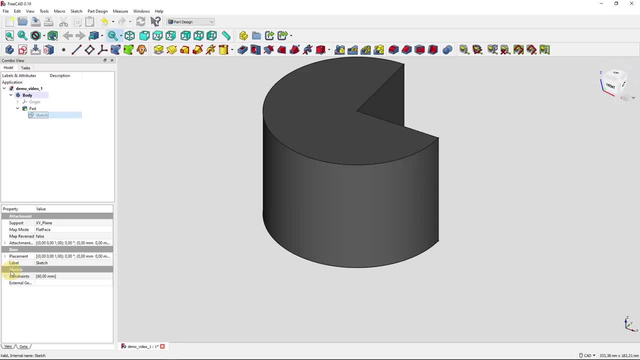 Or highlight the sketch here. Go to sketch constraints, Open it here And you see there is a constraint set to 60 millimeters And that's the radius of the sketch. So I can even adjust the sketcher constraints in my properties menu here on the left.